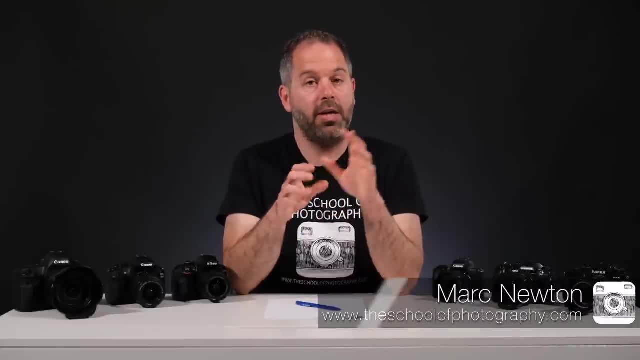 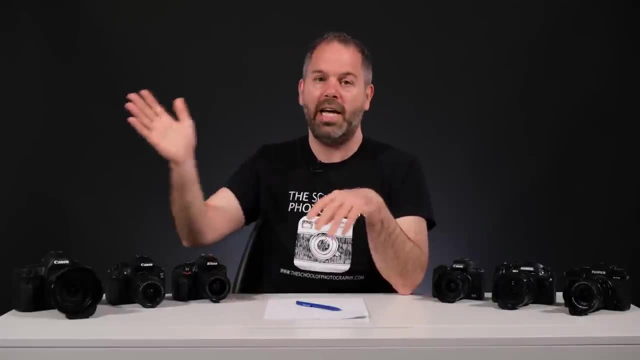 So you want to take your next step into photography and you thought to yourself: I'm going to buy a proper camera. So you've gone online. you're looking at cameras. all of a sudden you've got 10 tabs open in your browser and you are confused because camera A has got 57 focus. 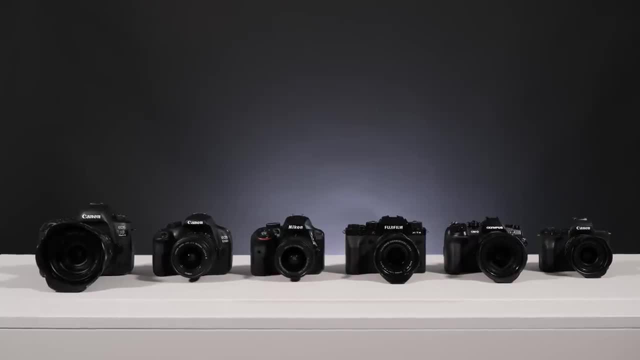 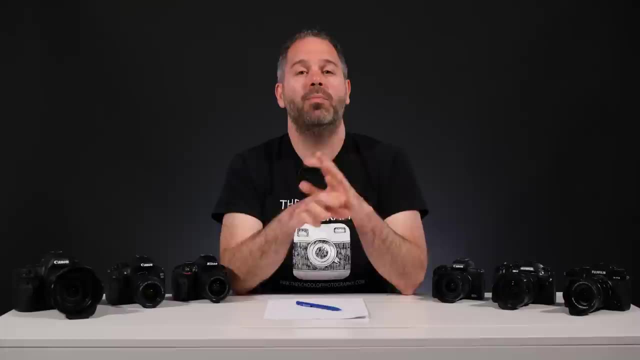 points and camera B has got 58 and you don't know which one is the best one for you. Well, in this video, I'm going to teach you how to choose your first camera, so by the end of it you will know definitely which one to buy. and if you are an experienced photographer, watching this, what I 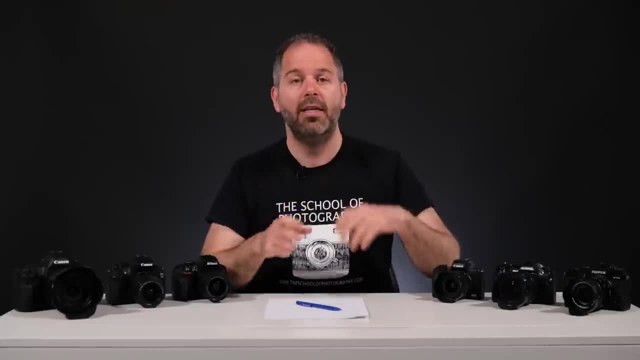 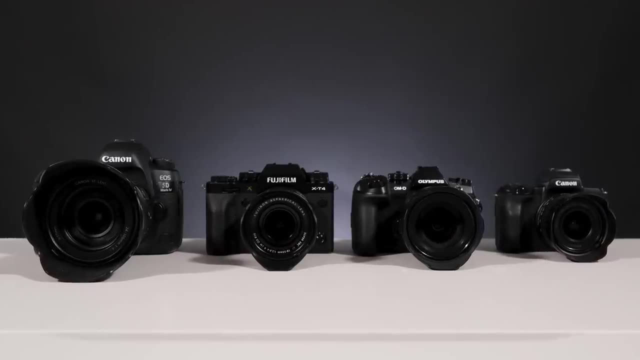 want you to do is put your experience in the comments so that you can help out all of these people that are looking to choose their first camera Now. I'm pretty sure the first thing that you are considering is that the actual brand to buy right Now. that is coming later in this video. 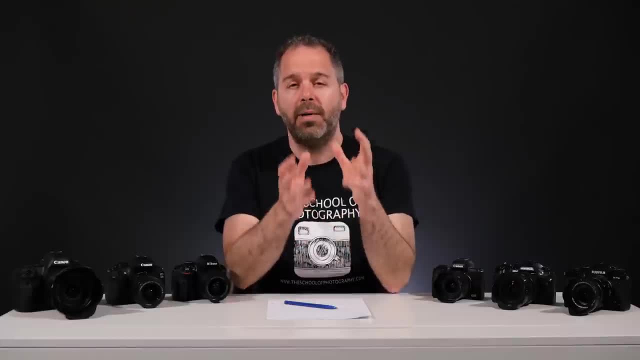 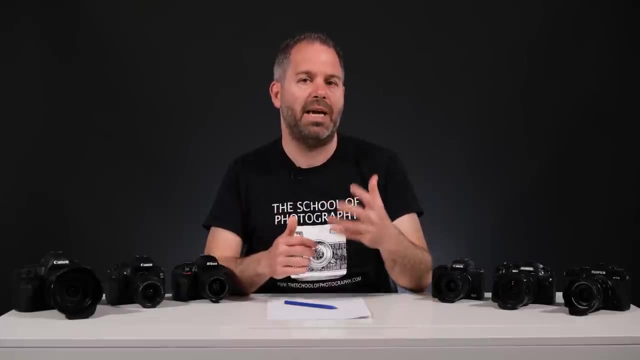 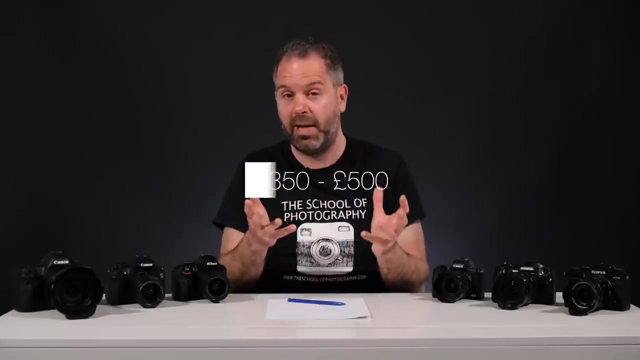 I've got lots of brands of cameras and we're going to look at that later on, but in reality, the first thing that you need to consider is your camera. How much are you prepared to spend? And it works out roughly like this: okay, for around 350 to 500 pounds you are going to get a real good. 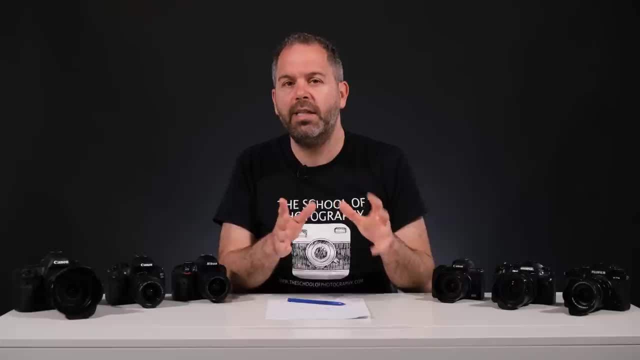 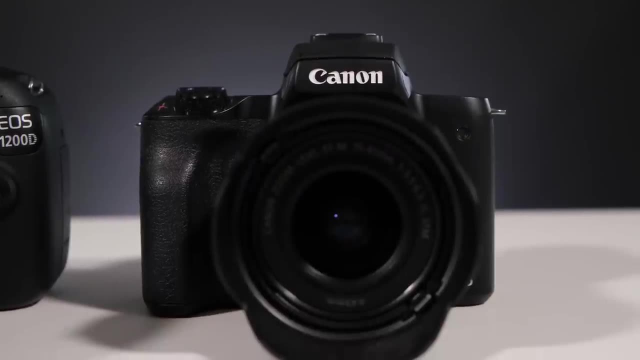 budget model of camera. If you increase that budget to 500 to a thousand pounds roughly, you're going to get a really good mid-range camera. and if you go above a thousand pounds and you can go on forever and ever, that's when you start getting into the real 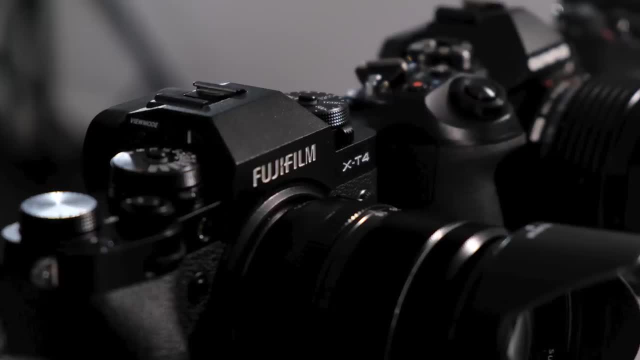 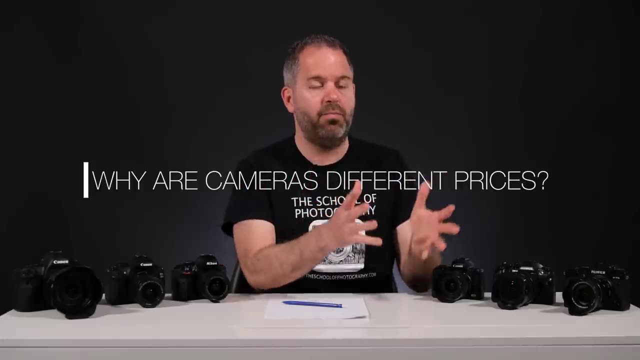 really kind of high-end camera models and you know the ones that are really expensive. So why are cameras different prices? you know why do you get a brand, let's say like Canon, and they have different price ranges of cameras. they have a budget option, a mid-range option. 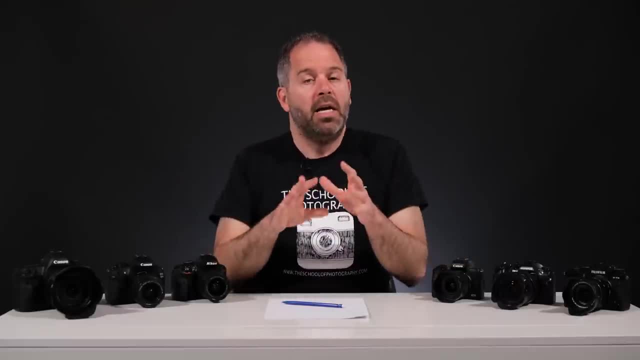 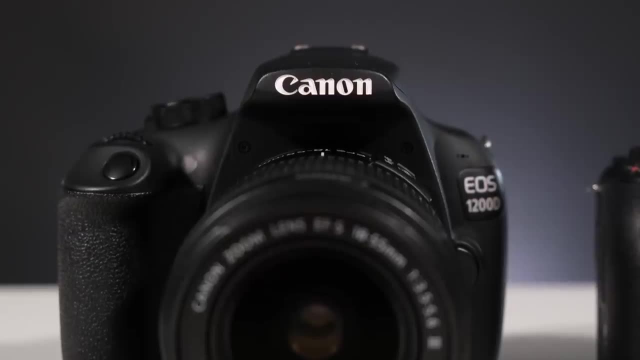 and a high range option. you know all brands do that. There is a few reasons why this is. the main one is build quality. so, for instance, down the lower end it's going to be plasticky, up the higher end it's going to be made of like metal and they're much more durable. 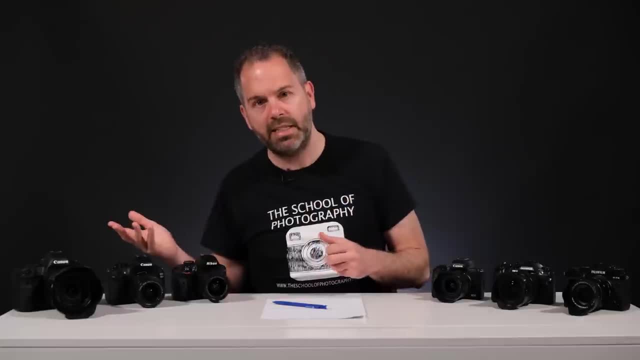 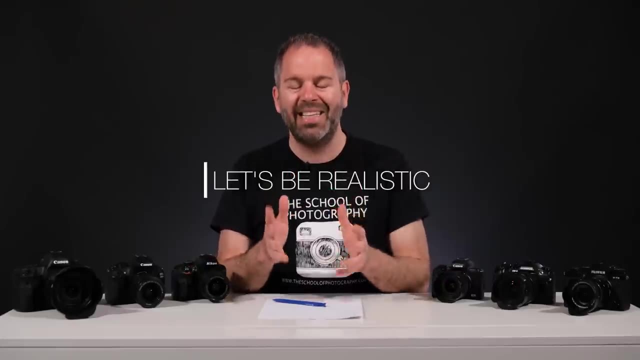 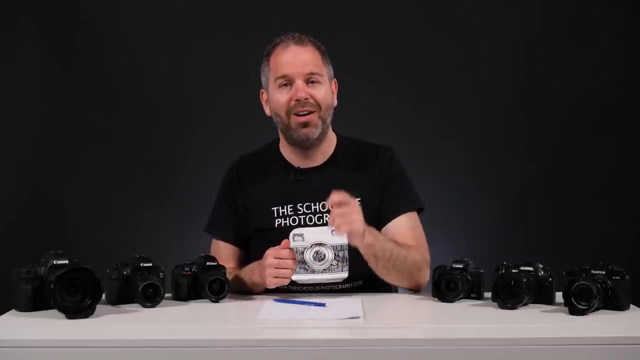 And then there will be features in the more expensive cameras that more professional photographers may use in their work. Now let's just break this down and be absolutely realistic. The more money you spend on a camera will not make your photography better when you are learning. it won't do it, I absolutely promise you. 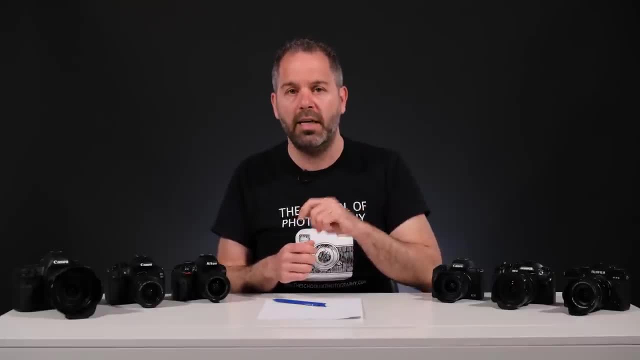 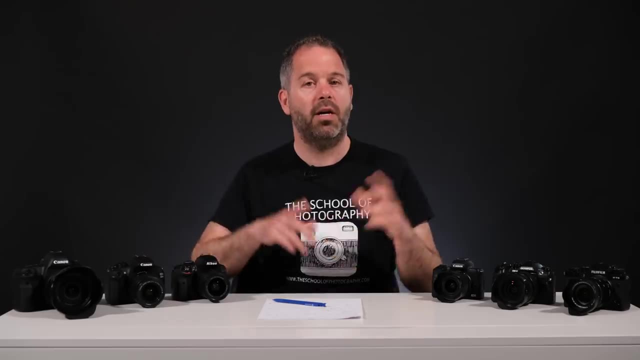 and an absolute fact is, if you can't take a decent picture with a cheaper camera, you are never going to be able to take a decent picture with an expensive camera, and I actually proved that in a video and I'll put a link to it should be coming across your screen now. go and 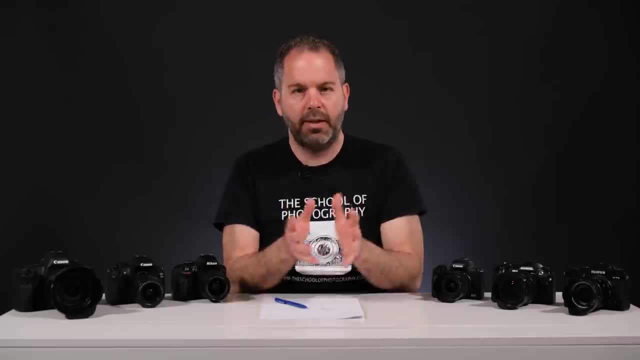 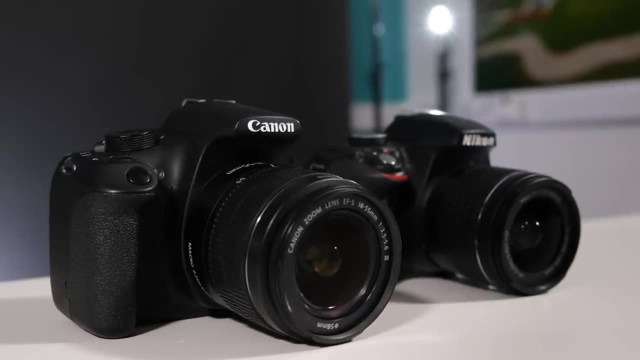 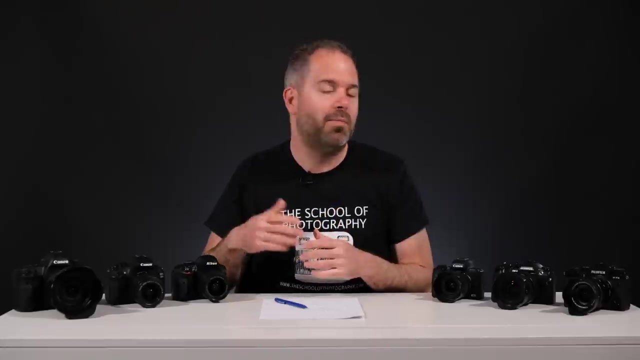 check that out. So to summarize there: think about your budget. is it between 350 and 500 pound? if so, that's the lower end budget range. if you've got 500 to a thousand pounds, then that will be a mid-range kind of model. then if you've got above a thousand pound to spend, you might want to go for. 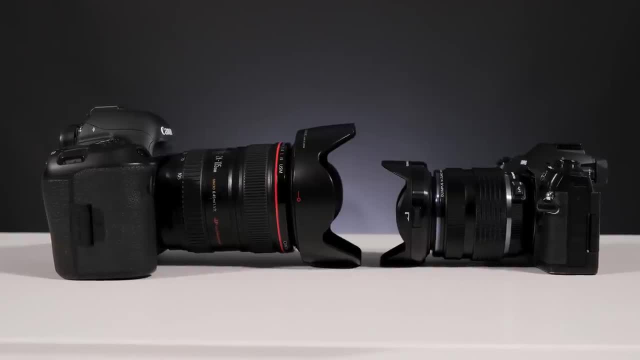 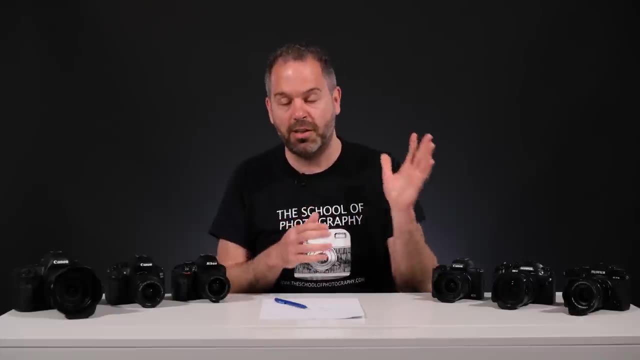 a higher end model. I wouldn't recommend it. actually, when you're learning photography, I think it's an absolute waste of money. I do know people that have got you know loads of money and they think to themselves: oh, I'm just going to spend it all now so that I've got a camera to. 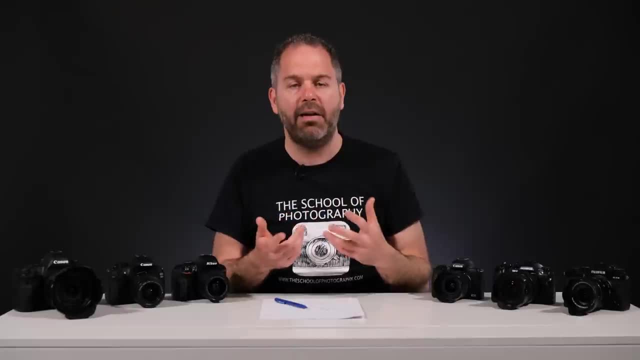 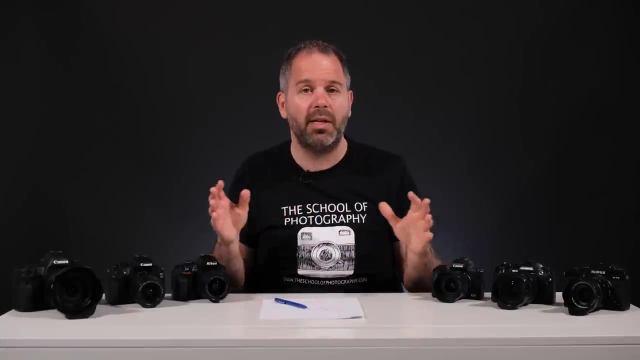 last forever and I kind of- and I do get that, I get that thought- but my recommendation for learning photographers is to start off with a budget model- and we're going to look at brands a bit later on- but it's to start off with a budget model because it's not going to make any difference to your 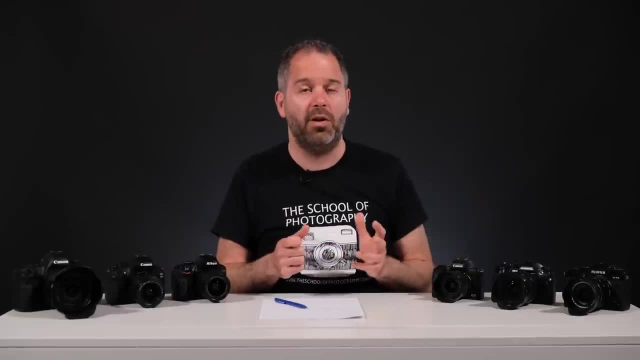 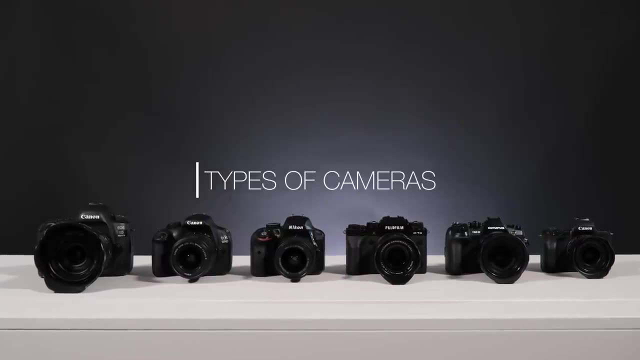 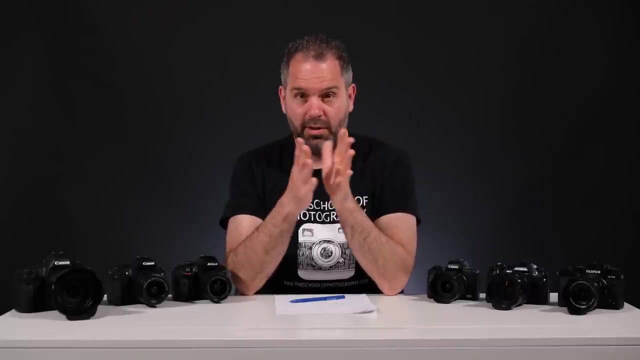 budget if you have a 2000 pound camera to a 300 pound camera. okay, so that's the budget. think about what you want to spend, and then you have to consider the type of camera that you want to get. right now. it basically breaks down to this: you've got compact cameras, which are the really small. 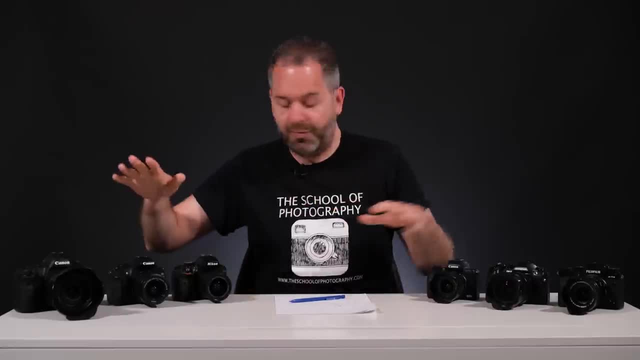 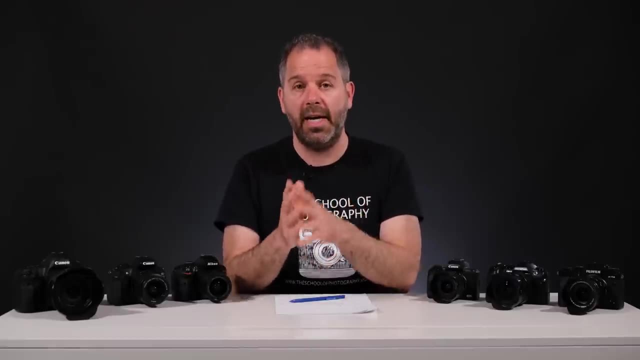 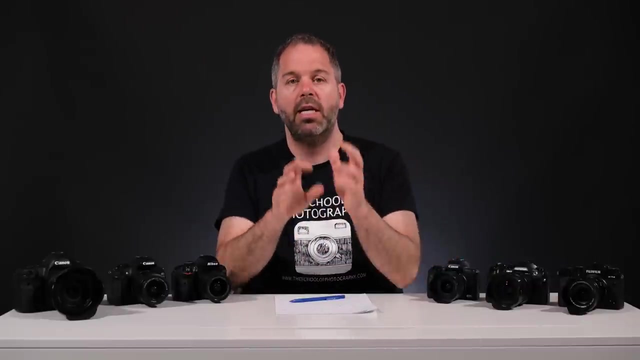 ones that you put in your pocket. you've got bridge cameras and then you've got these ones here that are dslr cameras. now, this one's really simple. all you will need is a camera goes to fully manual and a camera that has a lens that you can interchange if your camera 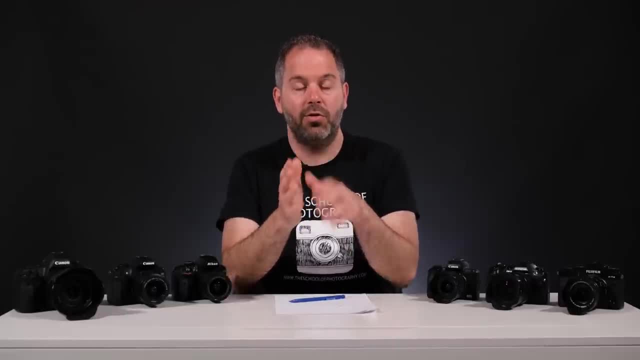 does that, then you've got the right type of camera to learn with and the right type of camera to control visual effects with. now, within the dslr range, you get mirrorless cameras and you get non-mirrorless cameras, and basically a mirrorless camera is smaller. it takes out the mirrors that 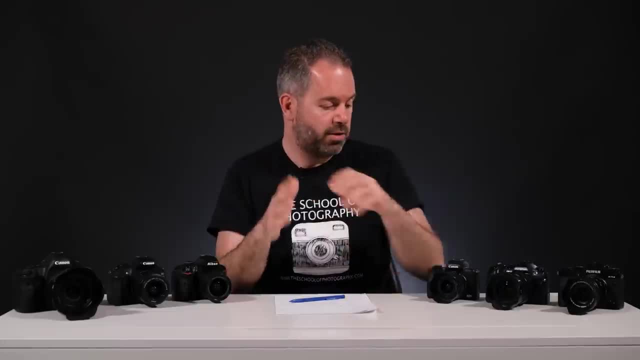 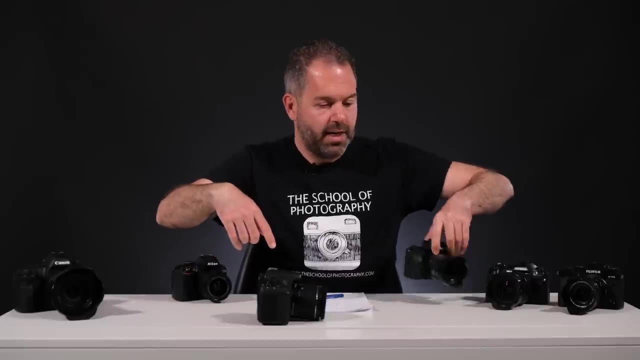 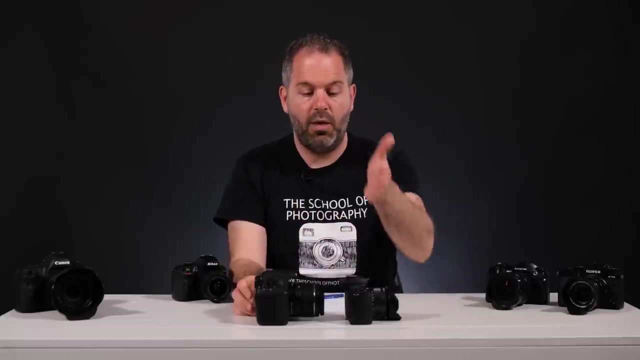 are inside the camera and it compacts the camera down to make it smaller. so i'll just show you that now. so what i've got here is two cannons: this one here is a non-mirrorless camera, and then this one here is a mirrorless camera. okay, now you can see, for then, two cameras, that one of body, this one. 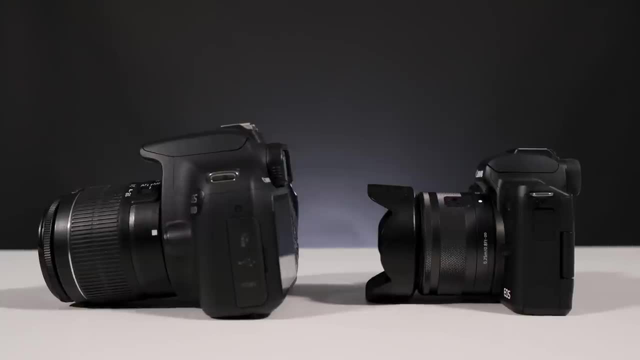 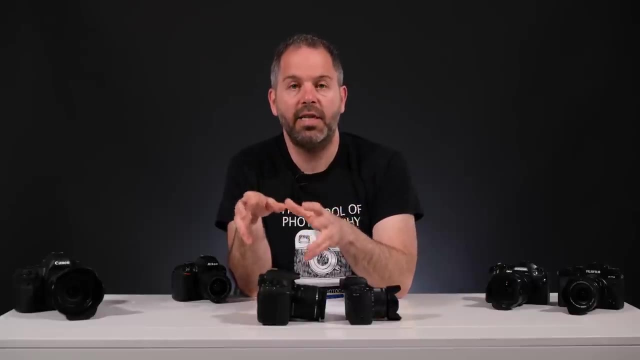 here. the mirrorless camera is a lot thinner than this camera here. now there is some pros and cons to it. a non-mirrorless camera, a camera with a mirrorless camera, is a mirrorless camera with mirrors within it- gives you live real-time viewing, so you're literally looking at the scene. 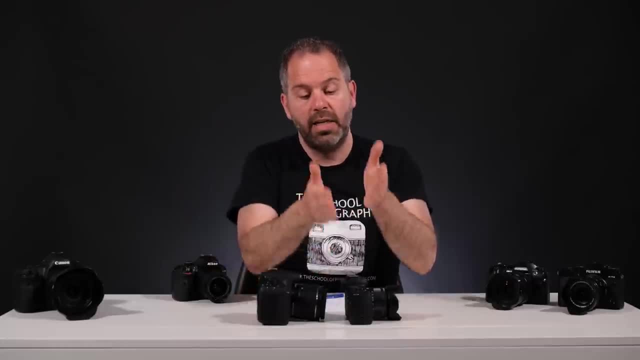 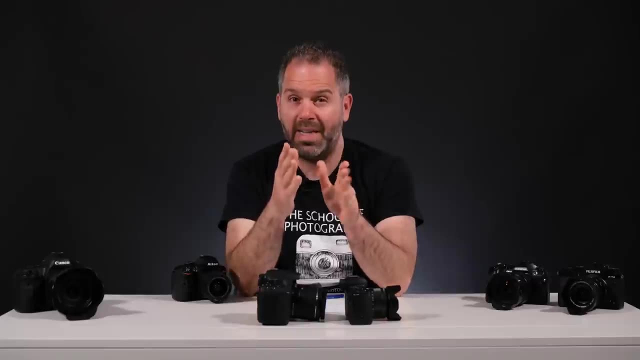 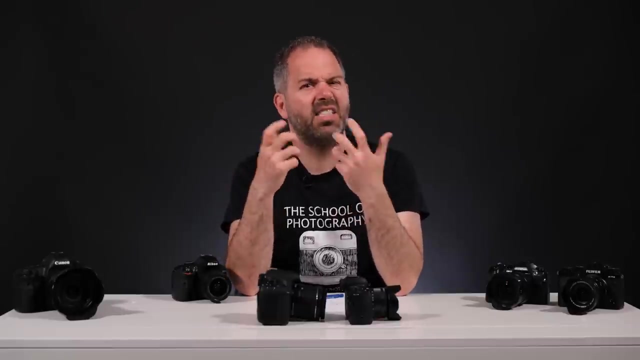 as it is, because it's just a series of mirrors whereas a mirrorless camera. you have to view the image either on the lcd display, which is problematic when you're outside, or you view it for a digital viewfinder and it's like looking at like a tv screen, if you like, and sometimes that. 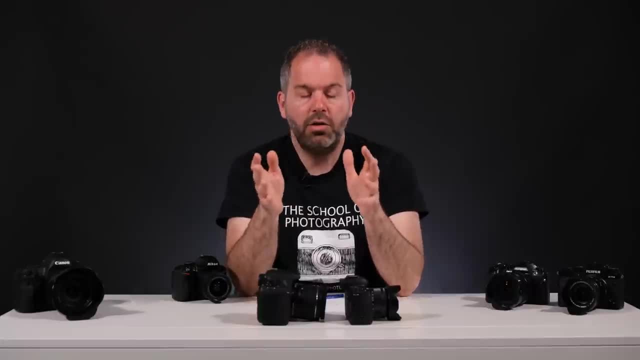 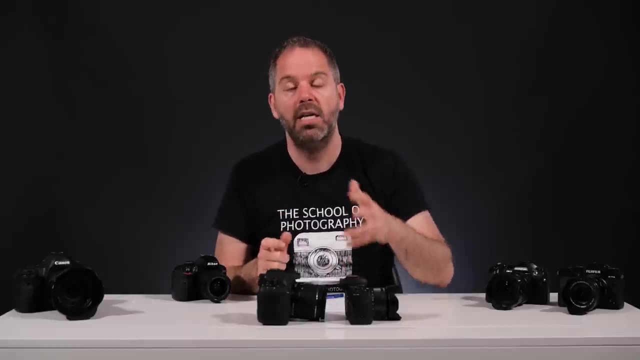 has a bit of a delay. so there are pros and cons to the mirrorless camera. the camera has a bit of a delay, but the mirrorless cameras are very, very popular these days and it is generally what people buy these days. but you still do have the option of getting a non-mirrorless one. they will also be. 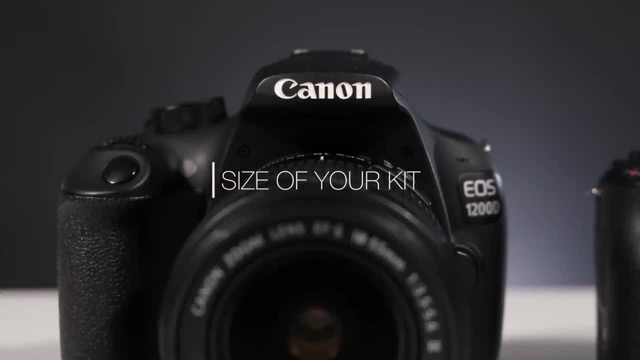 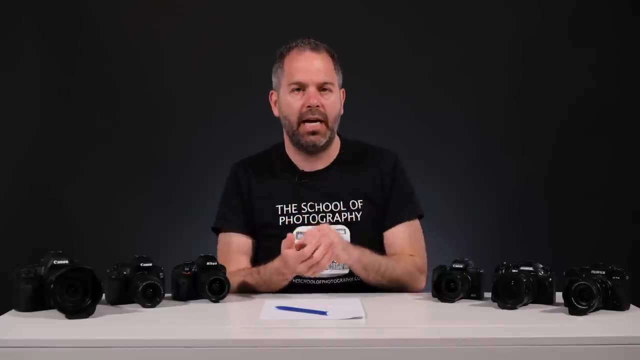 slightly cheaper as well. the next thing that you need to consider is size, the size of the camera. how much are you willing to carry around with you right now? you've got to remember that. it's all. it's not just to do with the camera. this is to do with the camera. it's not just to do with the camera. 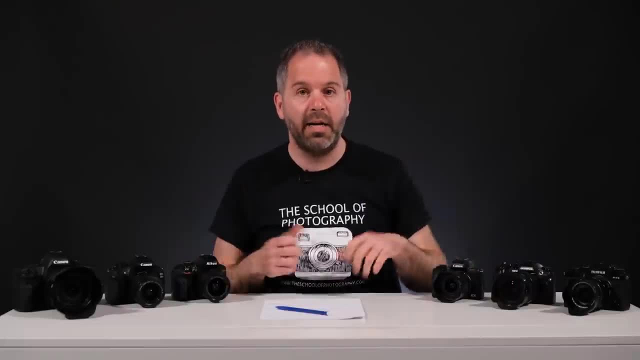 it's to do with the lenses, the tripod, the weight of things, the camera bag. everything has a relation to the size of the camera that you are about to choose and the size of the camera and its lenses and stuff like that. it's all dictated mainly by the sensor size which is inside the camera. now we 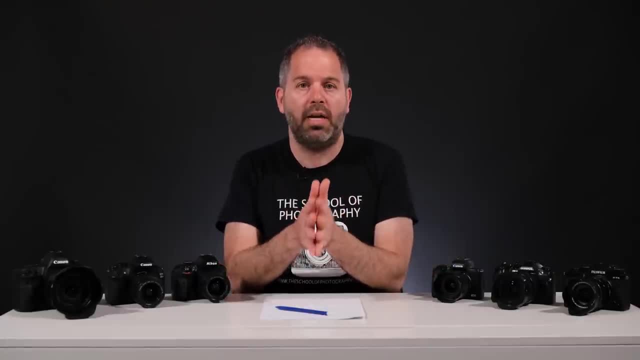 have got a whole in-depth video on camera sensor sizes. i recommend that you watch that because it gives you an in-depth view of what each one looks like and what you need to do to get a better view of what each one is and what they do. but just to break it down, a sensor is like a light sensor. 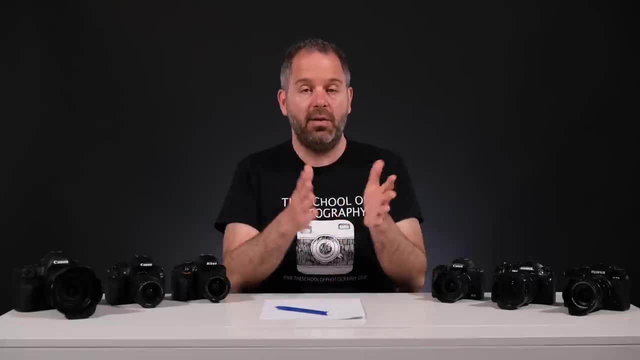 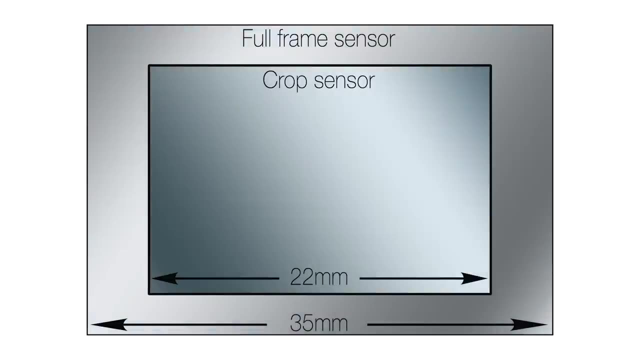 inside these camera bodies and that's what captures the light. and you have different sensor sizes. the common ones are a full frame sensor, which is quite a big one. then you have what's called a crop sensor, which is a smaller sensor, and you have a micro four third sensor, which is even. 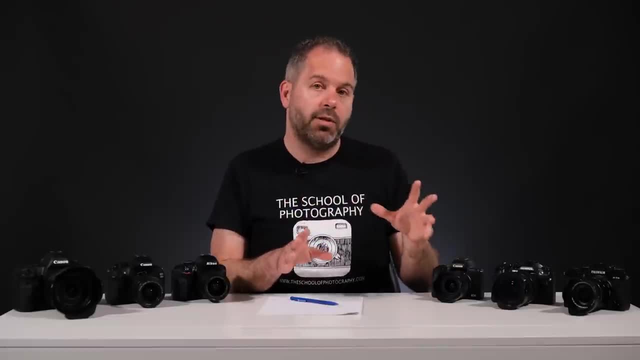 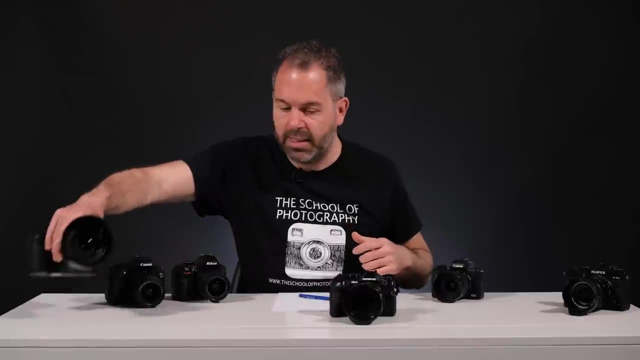 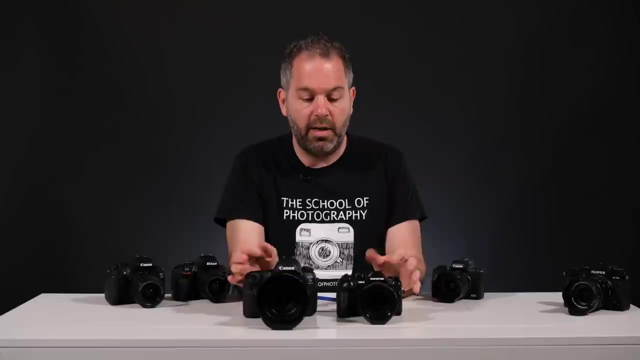 smaller still. so let's just look at the difference in camera sizes between a micro four thirds camera and a full frame camera, which is this canon one here. okay, now these two cameras, for argument's sake, are equivalent in the quality of the build of them, the features and all of that kind of stuff. 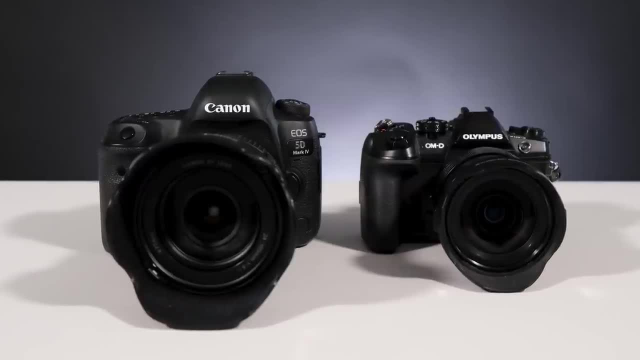 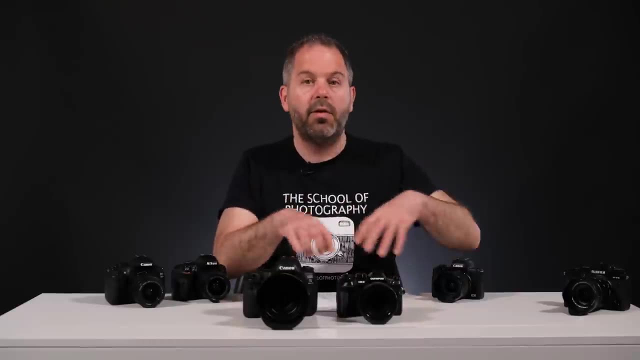 okay, the difference, as you can clearly see, is the size of the camera and the lens that goes with it, and the weight as well. and now let's compare that with a crop sensor camera, a sensor size which is in the middle. okay, which is? this one here and this one here, and this one here and this? 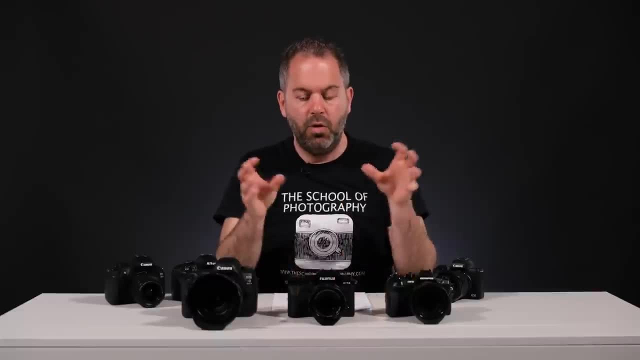 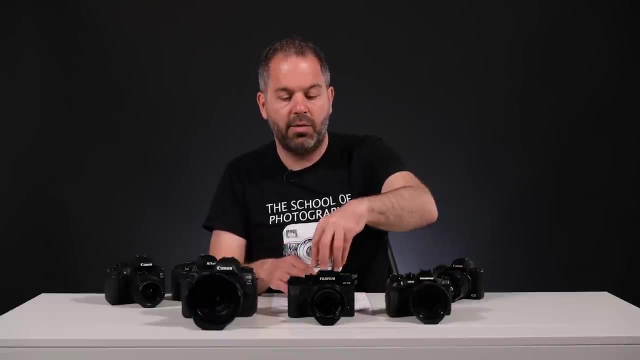 one here. we use the fuji for this one. now, if you look at the fuji, it looks very similar in size to the olympus. now this one's got a smaller sensor in, this one's got, for argument's sake, a medium sensor in, and then this one has got a full frame sensor in. okay, um, but you look at. 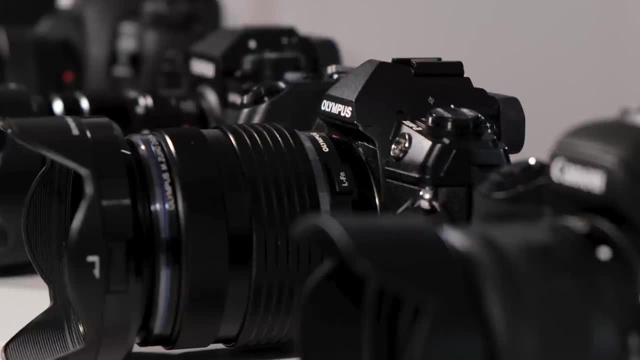 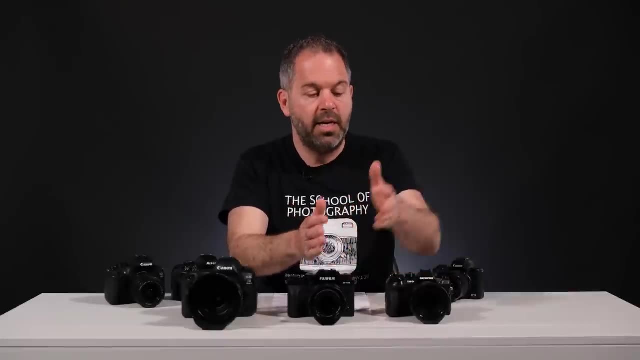 these two cameras here and they look very similar in size. but don't be fooled by that, because where it changes is when you start to put different lenses. on this crop sensor camera, the lenses are going to be a lot smaller and lighter on the micro four thirds they're going to be bigger. on 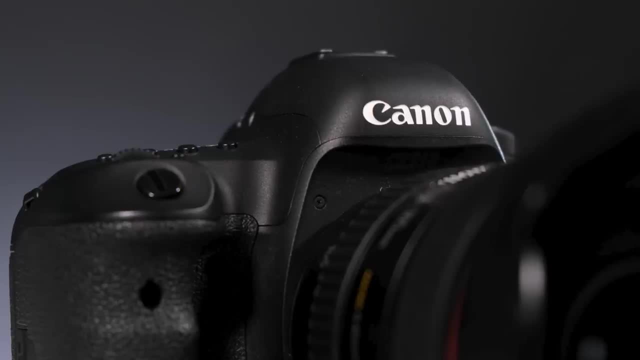 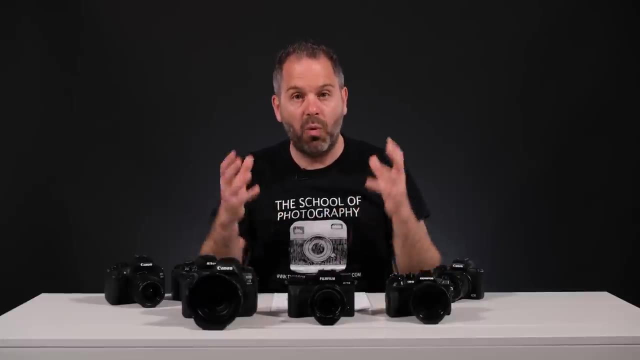 a crop sensor camera and they're going to be even bigger still on a full frame camera. and again, like i said, what you've got to consider is the weight as well, and then, with weight, you need a heavier tripod. so the heavier the camera, the heavier the tripod you're going to need, because it's all to do. 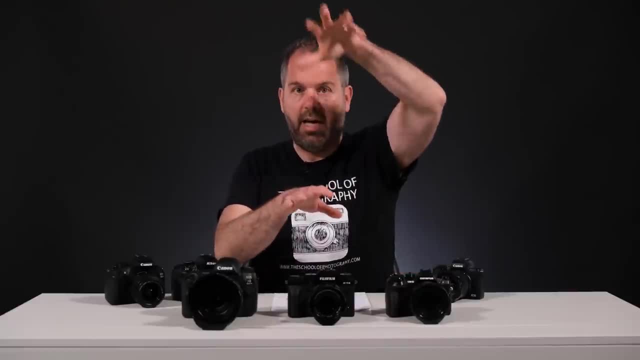 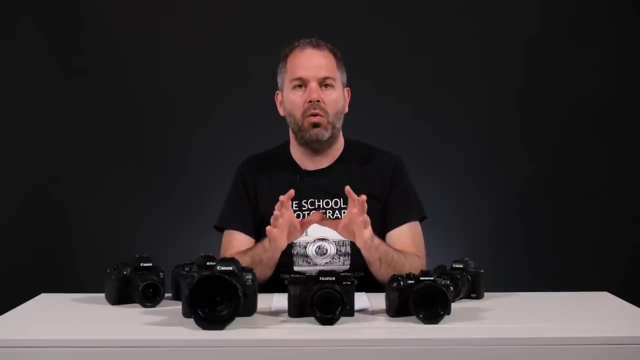 with physics, you know it's not rocket science. if you've got something heavy on top of something light, it's likely to topple over, okay. so you've got to think about that. you've got to think about all of these things when you are buying a camera. now there is an. 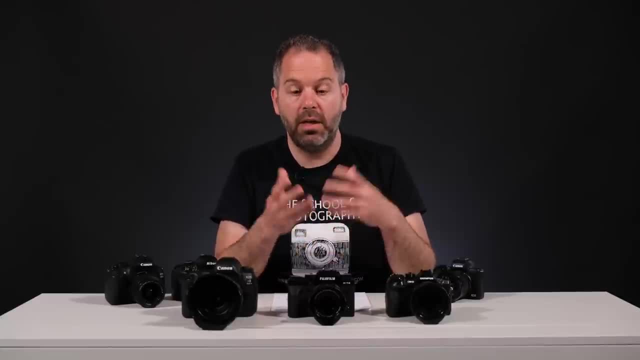 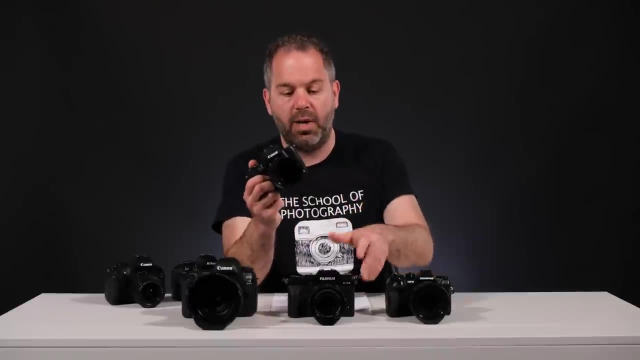 exception to the rule these days, because camera brands are building crop sensor cameras, that's, this size cameras in much smaller camera bodies like this one here. this one is the canon m50, right, so i'm going to move this along and put this one in the middle here, like that. 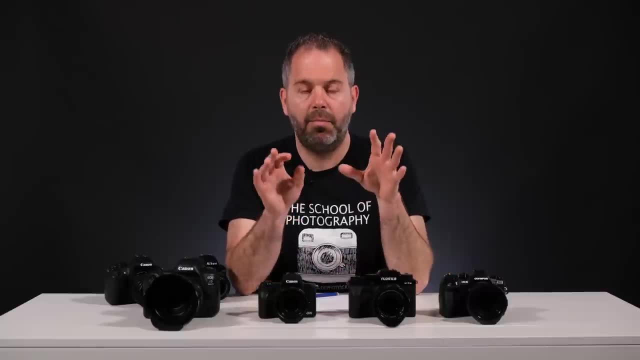 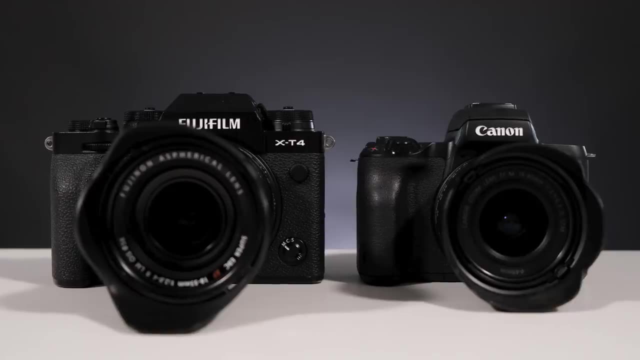 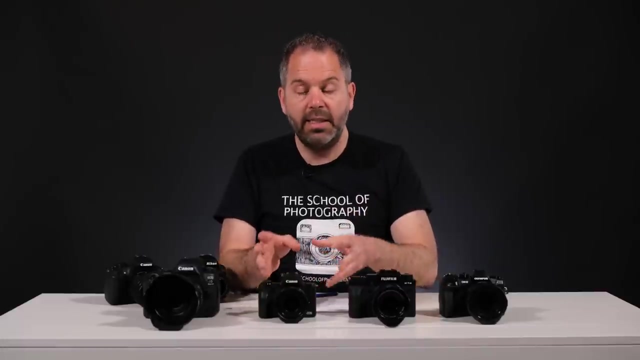 now these two cameras here, the fuji and the canon that i've got here. they are sensor cameras. they've got the same sensor size, but the canon here is a lot smaller. it's really small and really light and this is partly to do with the advancements of cameras these days. 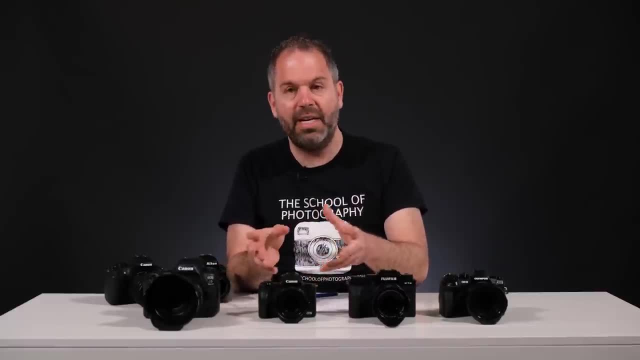 um, there is some cons to this. it doesn't have as many features that you can get to as quickly as possible, whereas these have. they're more professional, so you can get to all of the manual camera settings really easily, but still it's a very, very good option. 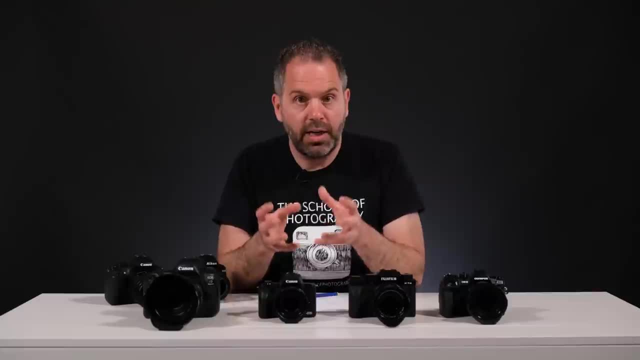 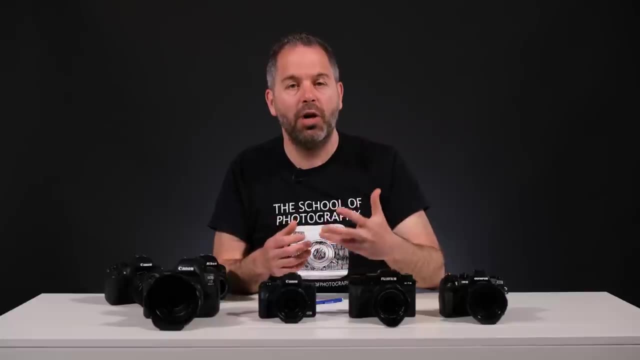 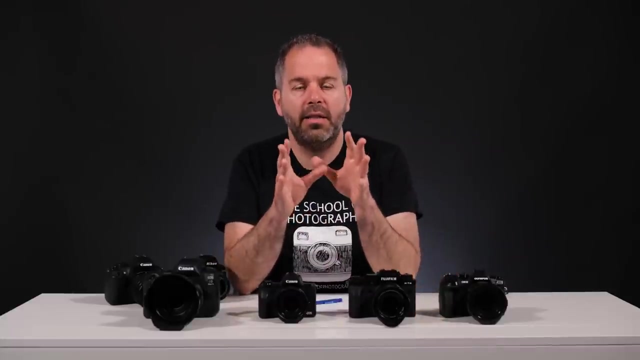 if someone is looking for size, they just want a really small camera. so now we need to talk about image quality versus what you're going to do with a picture, because that is ultimately what it comes down to when it comes to sensor sizes. the bigger the sensor size, the better the image quality will. 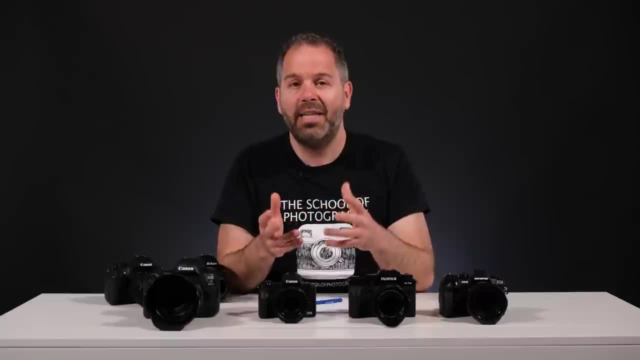 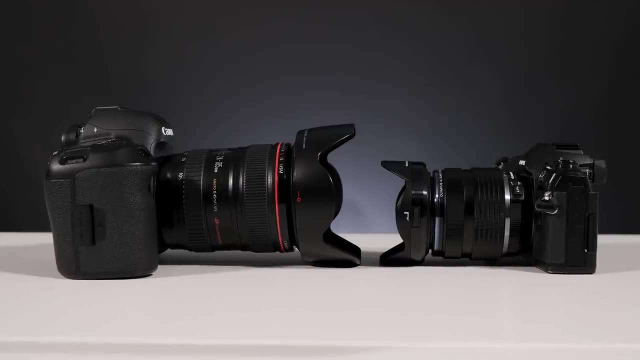 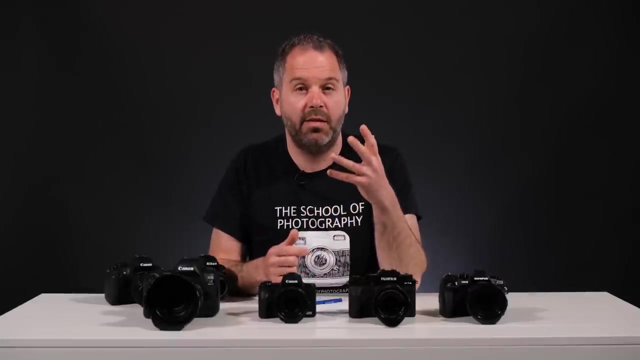 be, and it's as plain and simple as that really, and bigger sensors perform much better at higher isos trade-off to that, it is the size and the weight that you have to carry around. so you need to think to yourself what you're going to use the pictures for, if it is high-end advertising stuff or 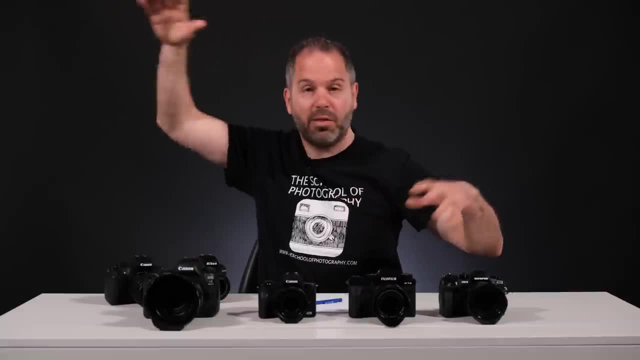 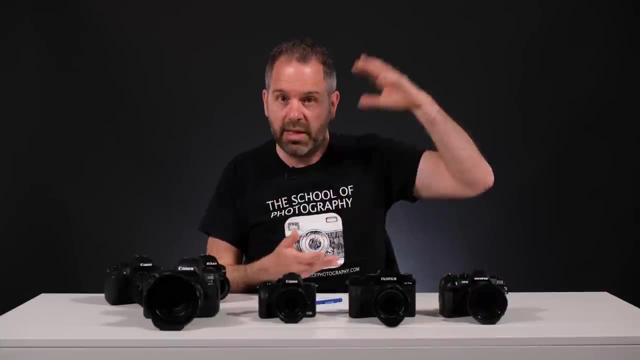 portrait photos that you're going to be printing, you know, as big as whatever. then you're probably going to need to go for a full-frame camera, because that's going to give you all the detail that you need to print the picture big, to retouch the picture and to give you what's called a higher 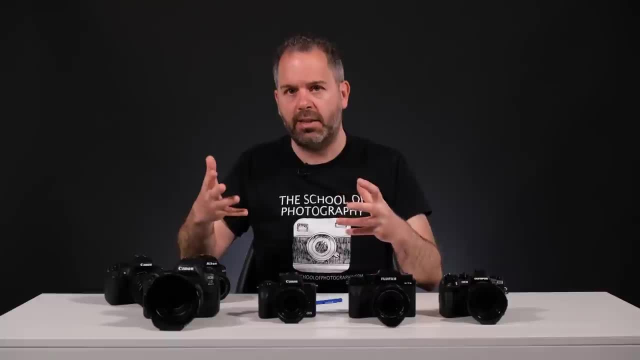 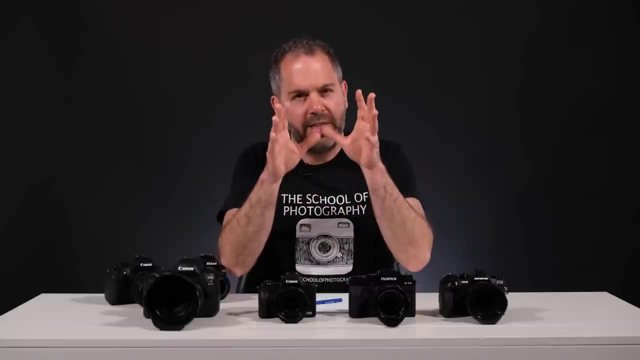 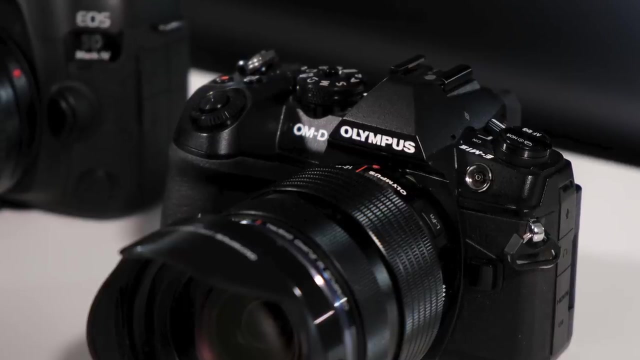 dynamic range. but let's face it, when you're learning photography, you're not going to be getting to that stage just yet, and you'll be surprised at the detail that you can get out of a crop sensor camera or even a micro four-thirds camera. they are so good these days that you can get decent quality out. 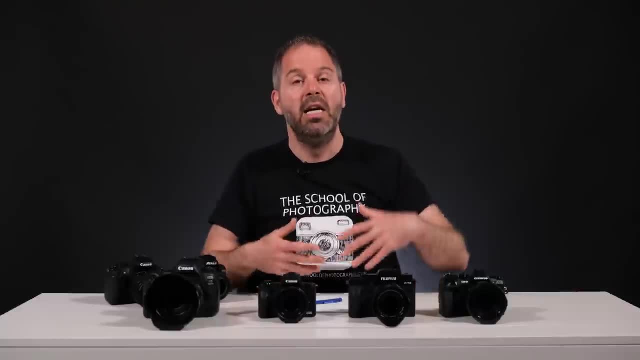 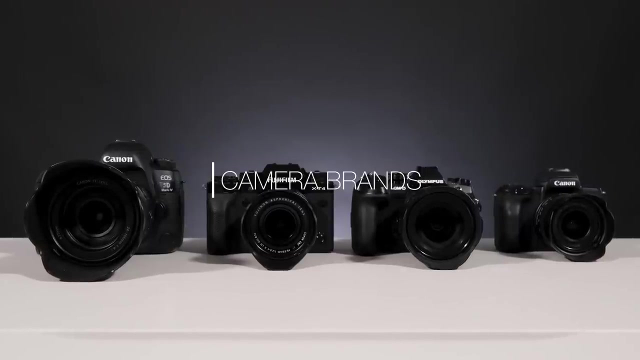 of any of these cameras, any sensor sizes. it's just when you are going to higher isos or printing big, that is when you are going to see a noticeable difference between the sensor sizes that you get. so now i'm going to talk to you about camera brands, but before i do i want to take this: 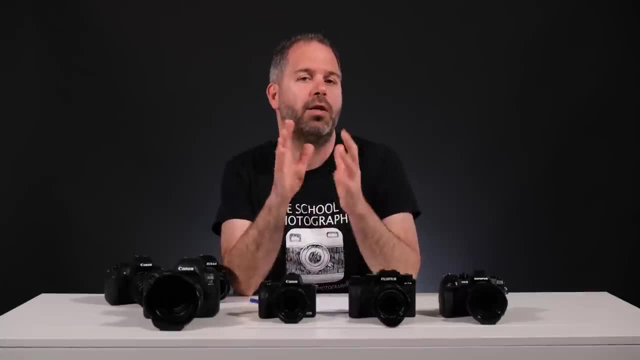 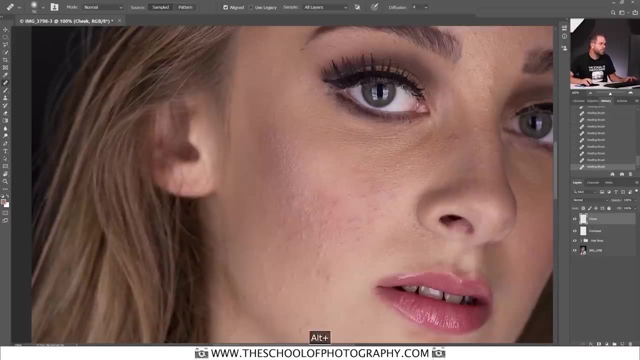 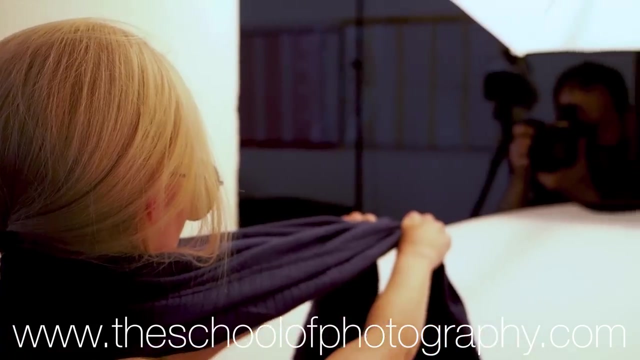 opportunity to tell you about the courses that we run over at the schoolofphotographycom. if you want to learn photography properly, we have got a structured professional photography course for you to come and check out. we are professional teachers. we've been teaching since 2002 and we've got tens of thousands of students all over the world. just go and check out our. 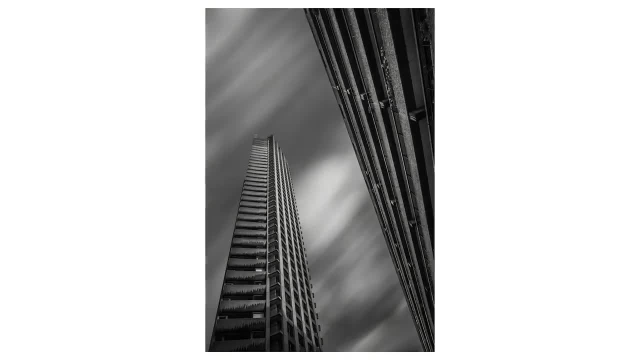 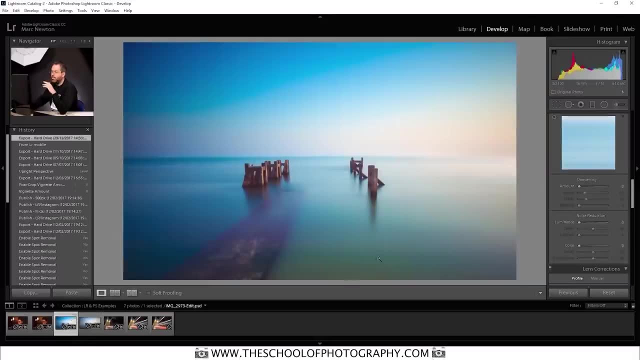 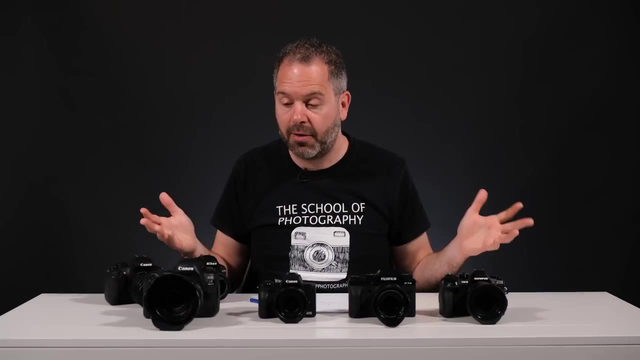 feedback on google and trustpilot and facebook and all places like that, all right. so if you want to learn photography or photoshop or lightroom studio lighting, anything photography related, come over and see us at the schoolofphotographycom. so let's talk about brands now, then, shall we? i'm going to 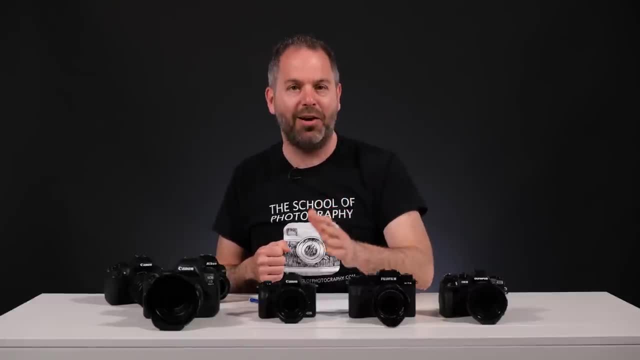 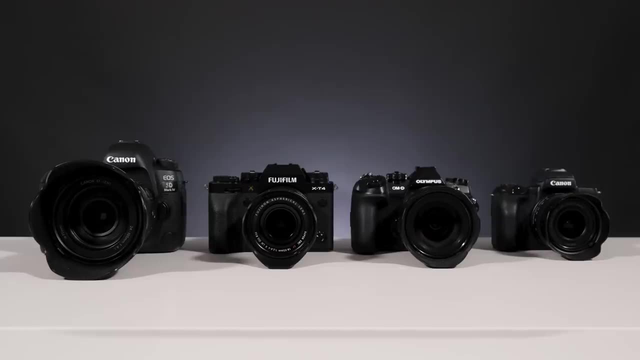 make this really, really simple for you. it doesn't matter, all right, i'm not getting paid by any brands and, incidentally, the reason i've got loads of different cameras here is because we get sent them. so we're very, very lucky, and these that i've put in front of you are really expensive cameras. 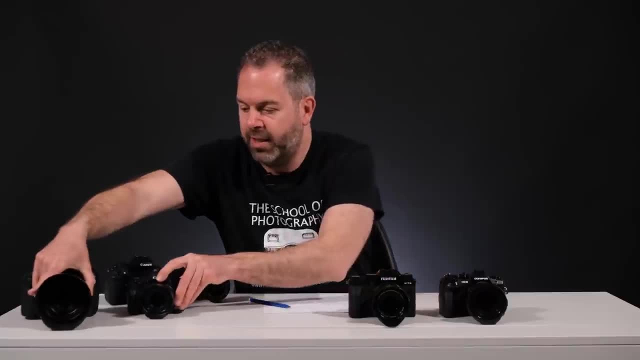 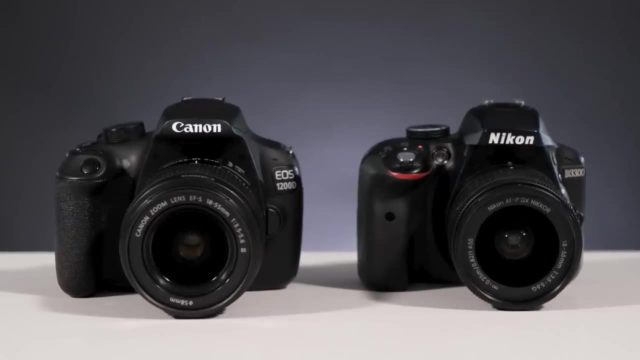 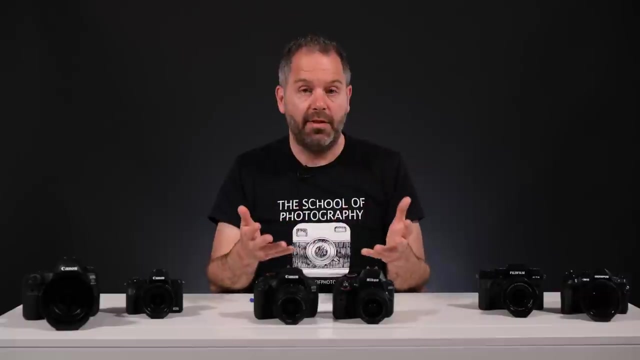 but i've also got these two here. let's just take a look at these. i'm going to move these ones out of the way. let's put these two here now. these are budget versions of common brands. as i'm sure you're aware, these are actually very old cameras, these, but it's the same thing, they're the budget. 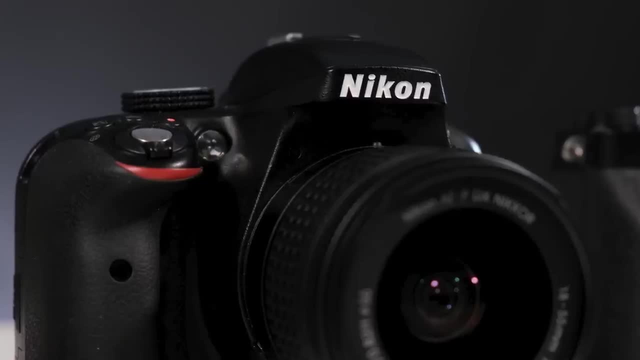 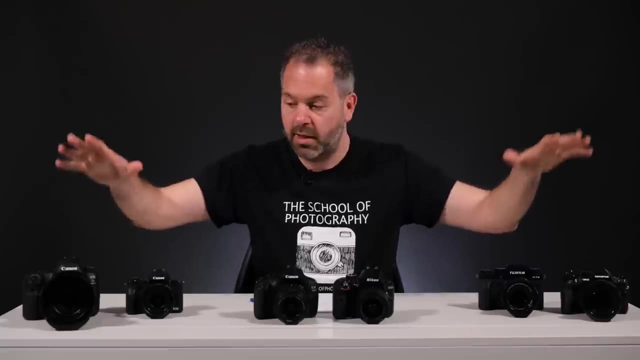 version, but maybe five years ago or whatever. and i want to repeat what i was saying earlier: if you can't take a decent picture with one of these, you are never going to take a decent picture with one of these, right? so it's an absolute fact. and the other thing i want to stress to you, right? 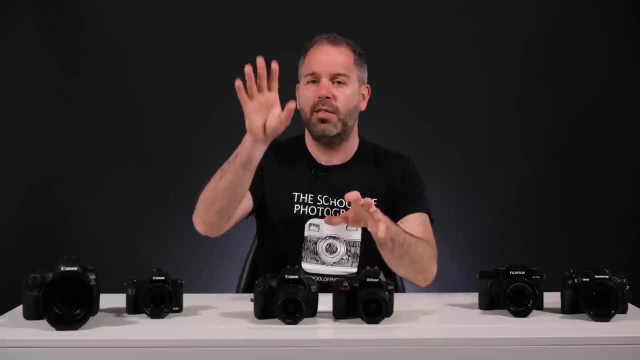 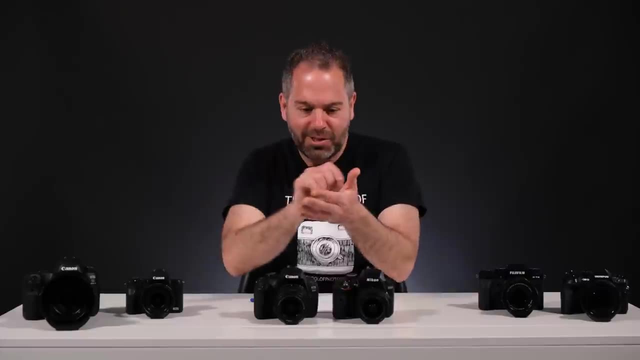 now is to not worry. remember, earlier on in this video i said that you've probably got six tabs or ten tabs up with all different brands of cameras and you're looking at all of the features and you're sitting there ticking them off and this and the other- all of them features don't matter. 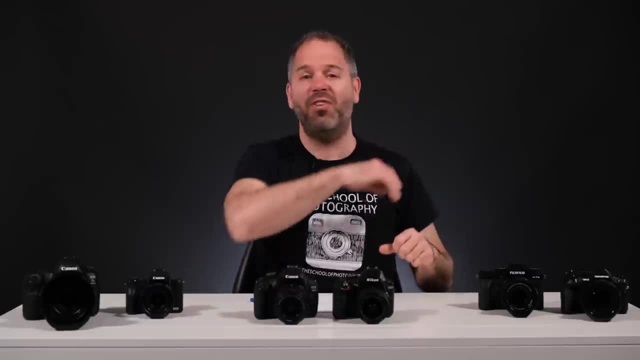 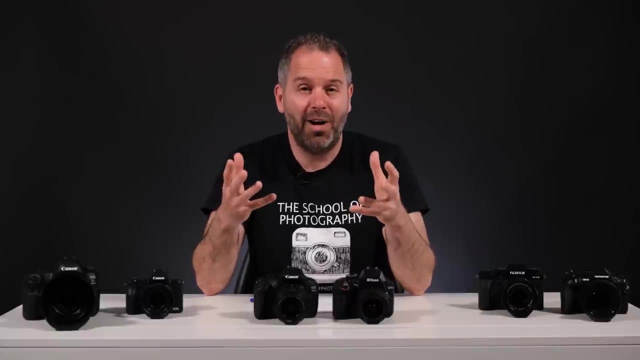 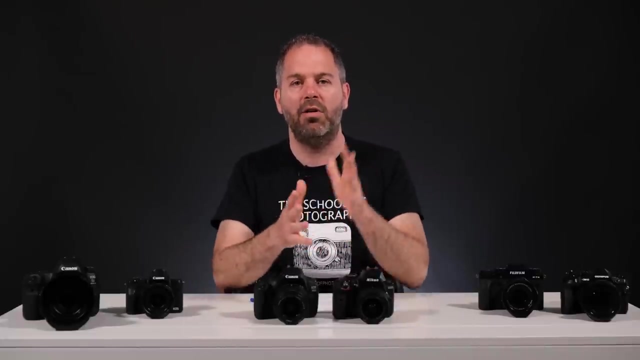 all right, the next camera brand will have the brand new feature that's going to compete against the next camera brand over here and they're pretty much useless most of them, right? so don't be sold by a brand new feature on a brand new camera. it's not going to make any difference to your 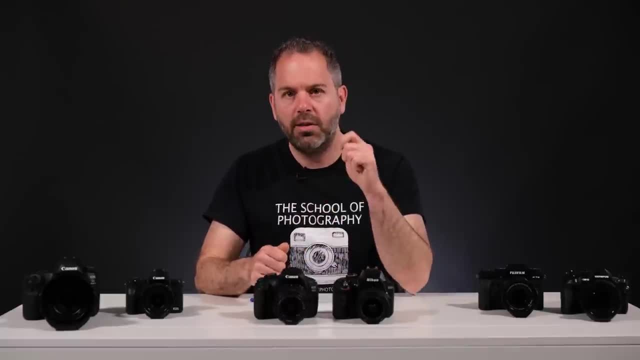 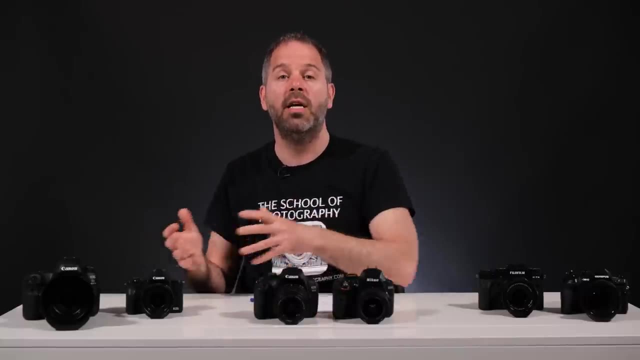 photography and to your learning of photography. what i do suggest, though, is that you choose a brand that maybe friends and family are using, and the reason for that is you can pick the phone up and ring them up and say: oh, what's this button do, or can i come out and 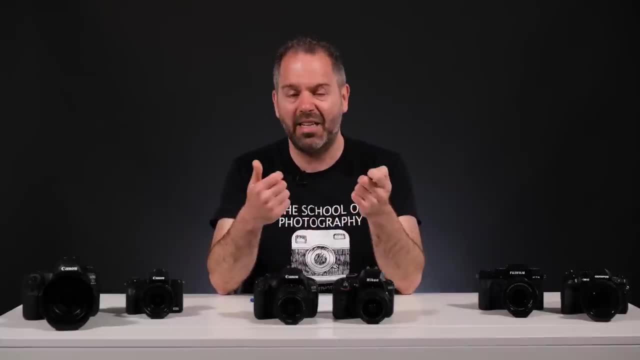 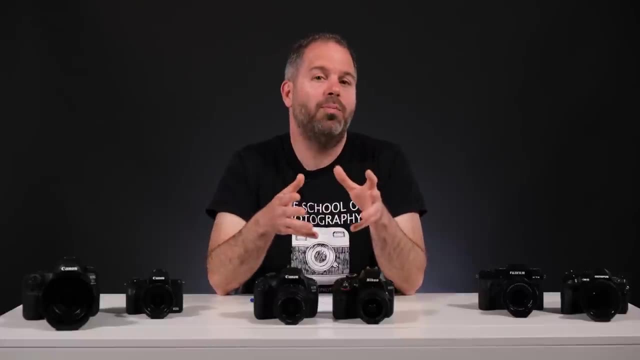 shoot with you and you use the same camera brand, it's going to be easier, right? so if you're choosing a camera brand that a more experienced photographer that you know has got, it's going to help you out in the future, but not one of them is going to make your photography. 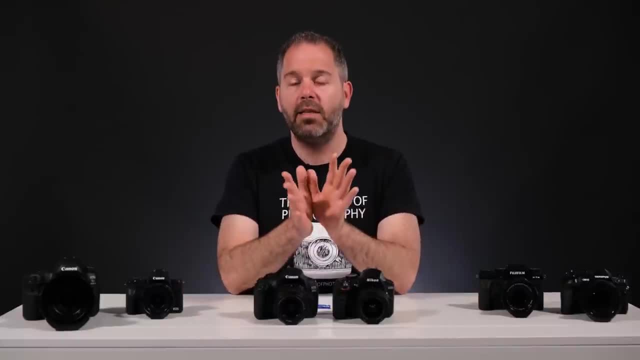 better than the other one. i can promise you that the next thing that you might want to consider is filming. if you're not planning on doing any filming, then you have to worry about this section. It's very popular these days vlogging YouTube videos. 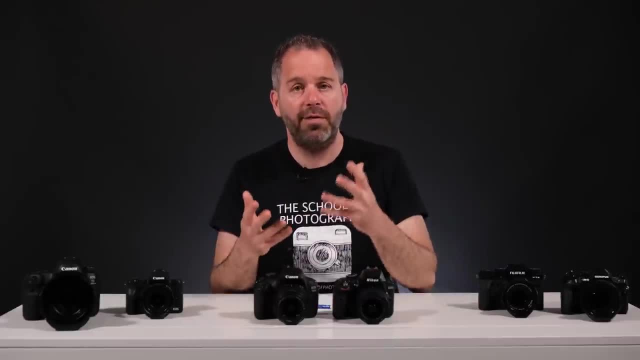 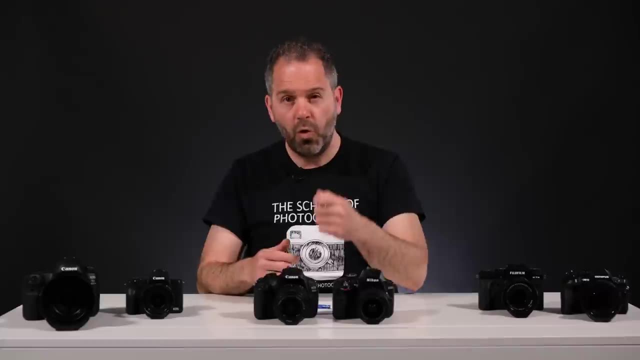 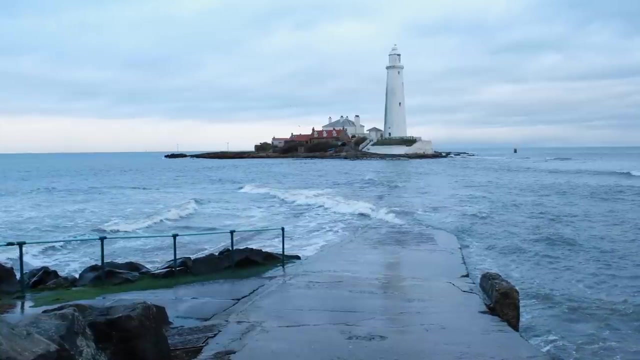 whatever, and cameras do a great job at filming. Now here is my advice here: Try and choose a camera that films in 4K and, if possible, it films up to 60 frames per second, because that allows you to slow the film down. 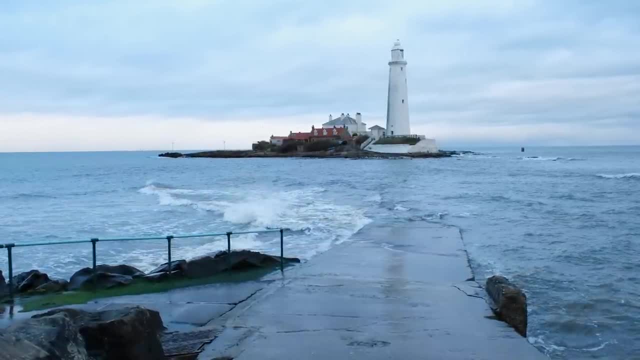 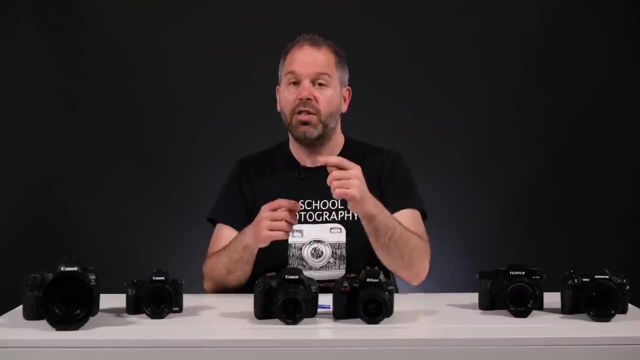 and that looks really cool in videos. The 60 frames at 4K is not essential, but if it's there, I think it's a really good feature. So make sure it's 4K for a start, and if it's got 60 frames per second at 4K. 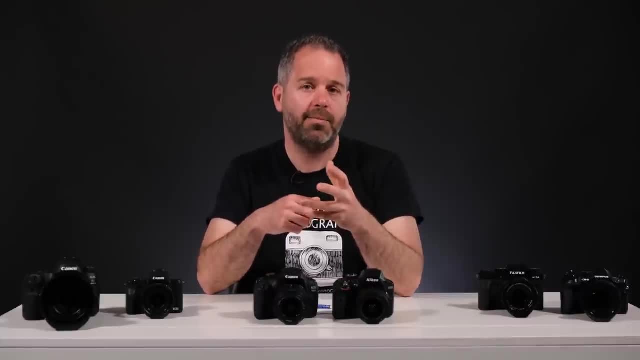 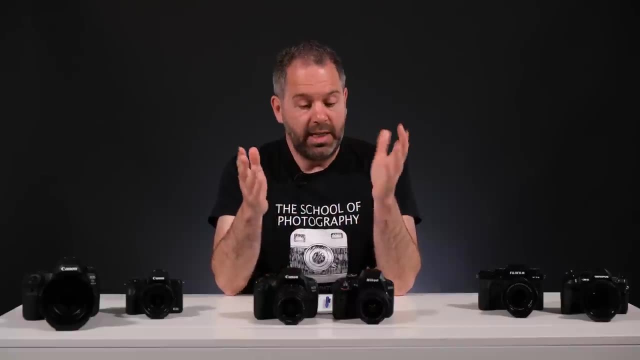 then I think that you've really got a good filming camera. Now, what about secondhand? What about buying secondhand equipment? I think it's a really good option. You can get these cameras here, I'm pretty sure, for about a hundred pound now secondhand. 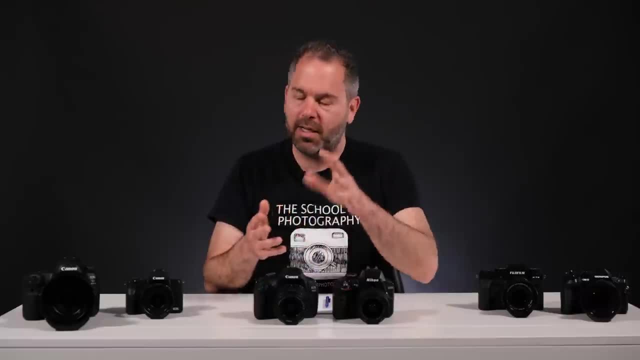 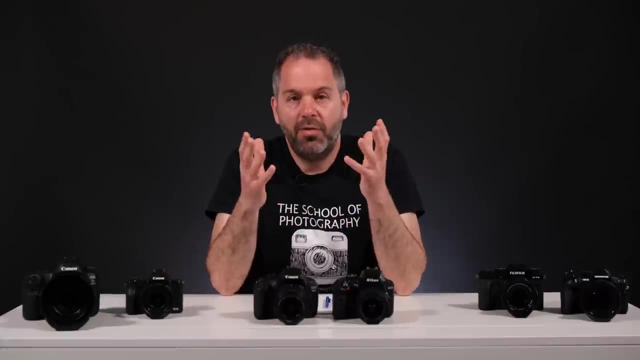 and that is an absolute bargain. And, like I keep saying, you're gonna take the same picture with this to start with as you would with that one. So if you're interested in buying secondhand, I think that it's a really good option to go for. 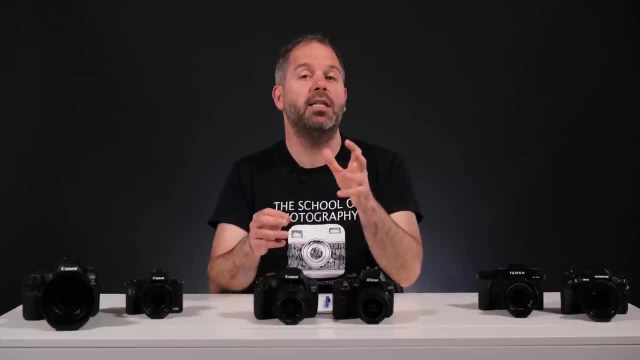 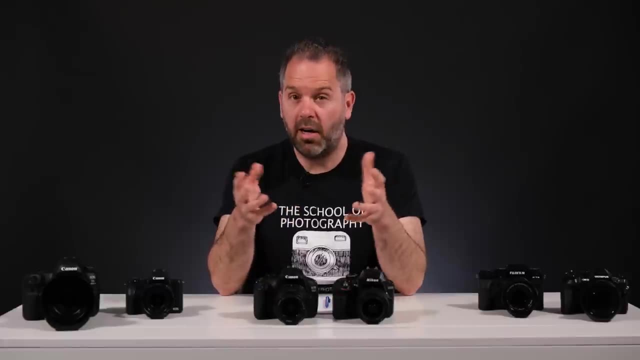 but it can be risky and these are the things that you should be looking out for. Try to find a camera that's got a low shutter count. So, just like a car, when you have mileage, and you buy a car if it's got high mileage, you know it's been used a lot. 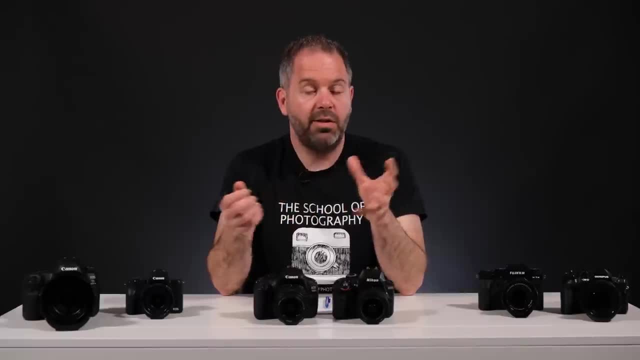 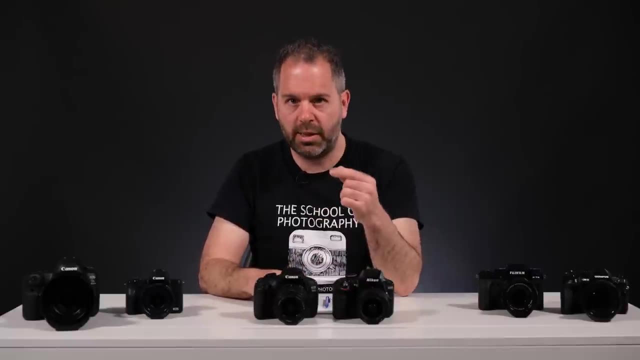 Cameras have shutter counts and they're very easy to find. You just plug them in to software and blah, blah, blah, you get the shutter count of the cameras. So try and find one that's got a low shutter count And, if you can, 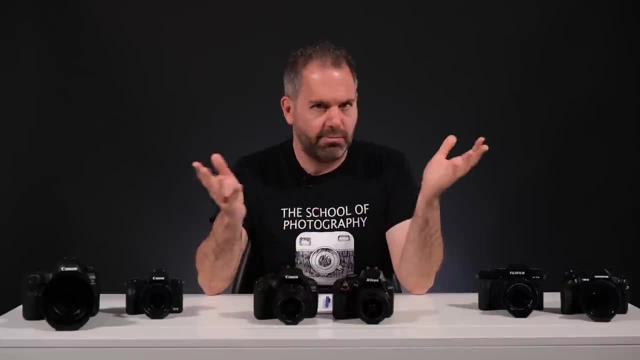 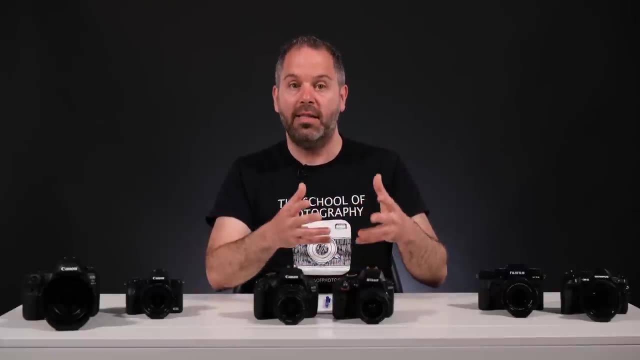 try and find out the history of the camera. Again, let's take the buying a used car scenario. You know one previous owner. If your camera that you're buying is with one previous owner, you know the person you're buying it off. 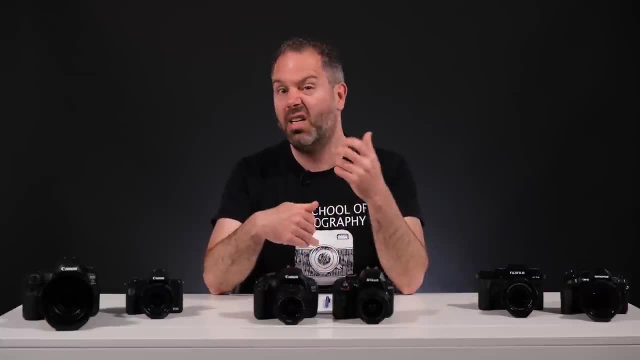 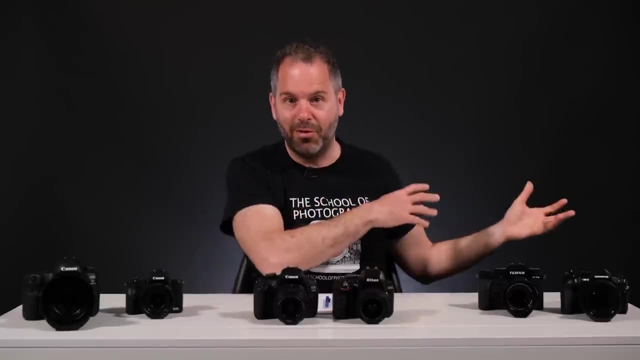 was the first person to buy it and use it And it's got a low shutter count. you're pretty much gonna get a decent camera. If you're buying it off, doesn't know where it's come from. you know they've bought it second hand. 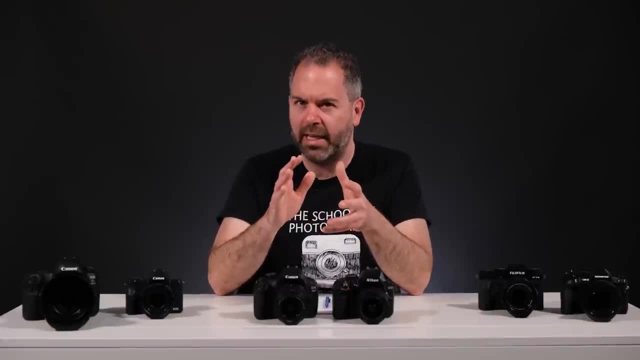 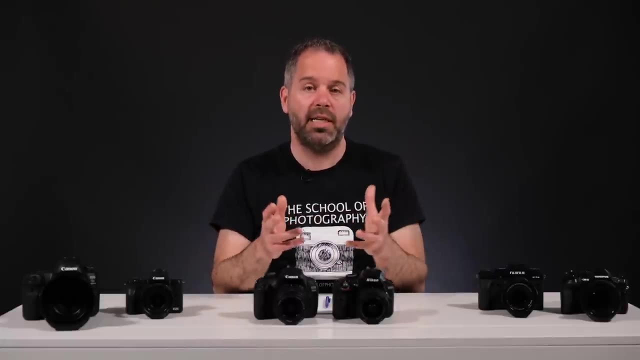 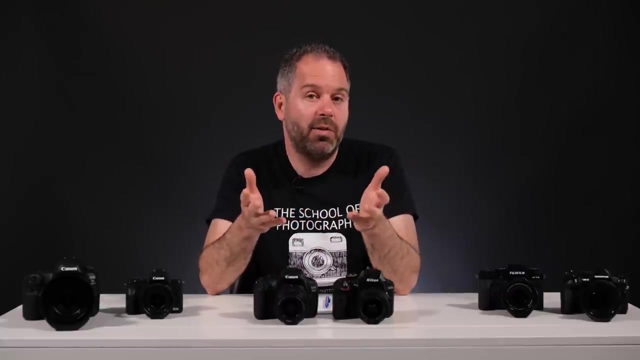 themselves. you might want to, you know, start rethinking that. the other thing that you can do is go to well-established camera selling companies. you know online companies, shops etc. and normally they have a second hand range and them cameras would have been looked at by their experts in. 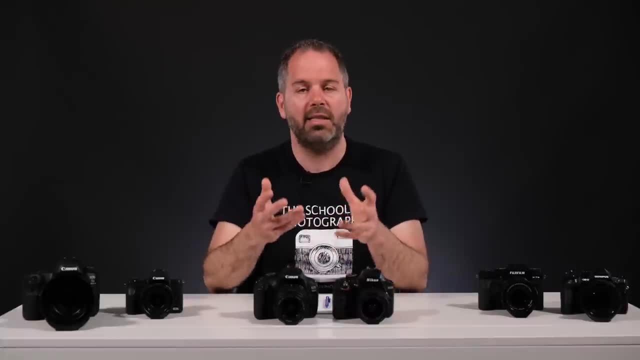 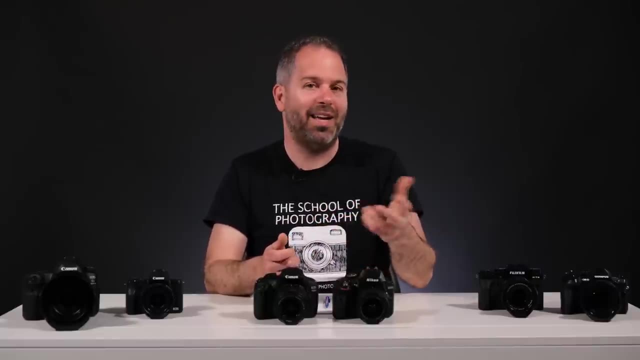 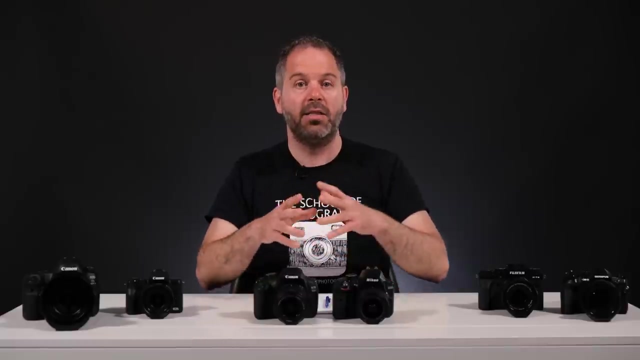 the shop so they would have been taken apart, tested, cleaned etc. so you've got half a chance of getting a good one there, but they will be dearer than what you would pay on an internet auction site. and then you have refurbished cameras that you buy second hand. so camera brands like 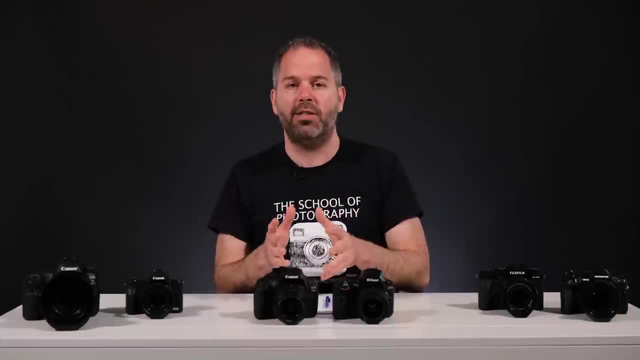 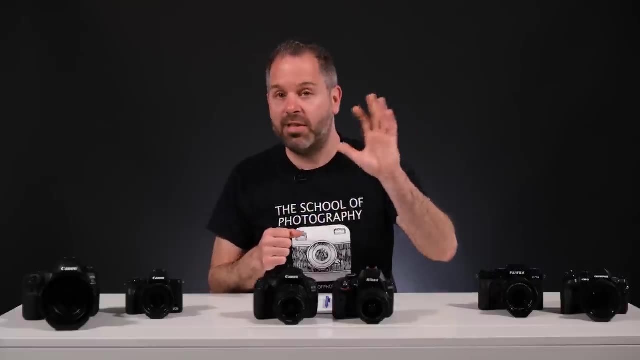 fuji, etc. they have a refurbished section. now what that is is it's where people have bought a camera from their shop and have sent it back, and they might have sent it back because it had a fault. they might have sent it back because they just didn't want it anymore. the problem there is you. 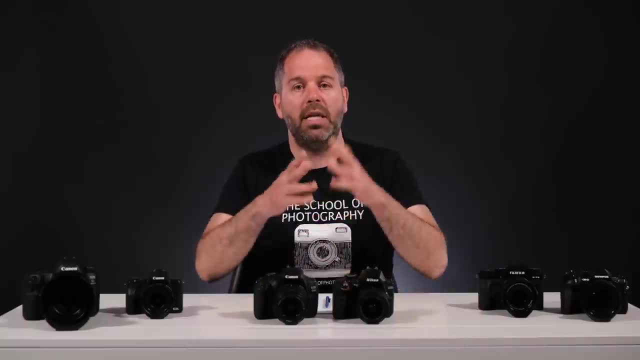 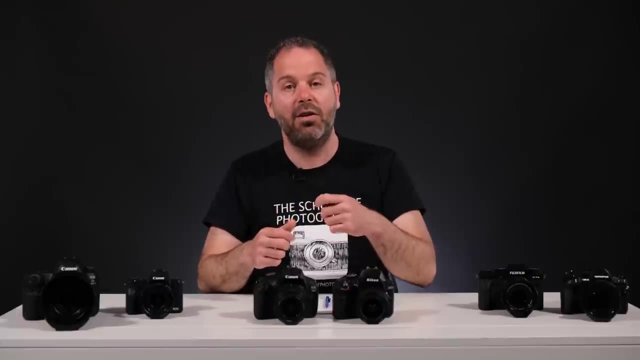 actually don't know that, but what you do know is that the experts at their factory or wherever it goes back to they have checked through the camera. they've made sure it works, and you normally get a year's warranty again if you buy a refurbished camera. so that is another option to get a slightly lower cost. 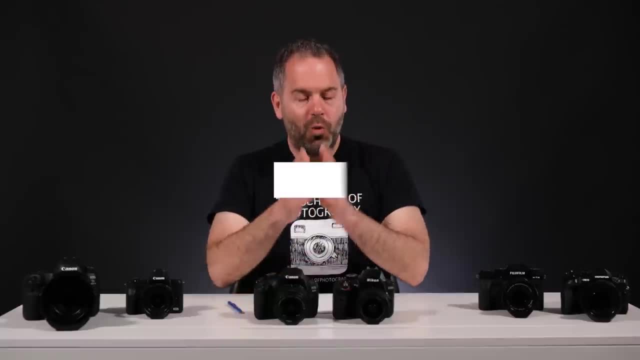 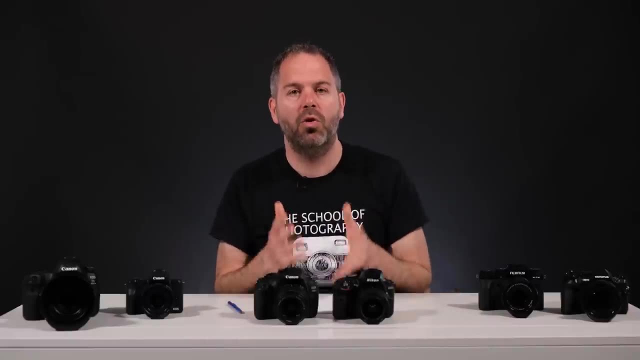 camera. so let's just do a recap on what you should be looking for when you are buying your first camera. firstly, your budget. think about how much you want to spend on your first camera. if you're thinking about how much you want to spend and stick to it, okay, stick to your budget. when you're 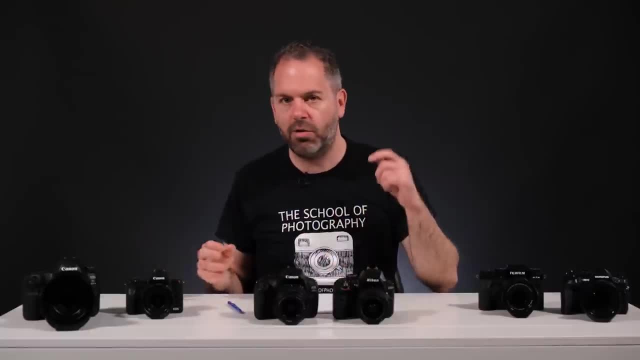 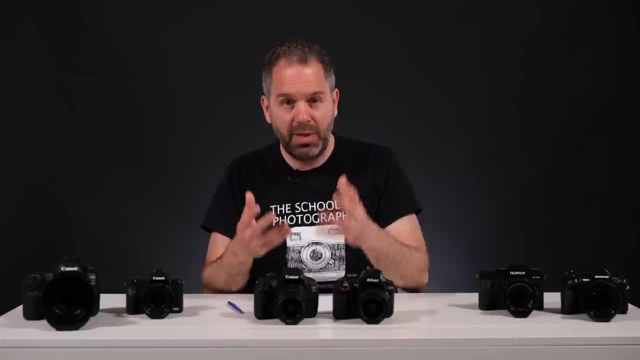 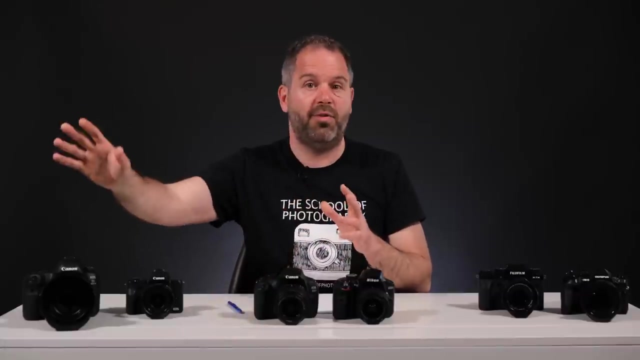 starting in photography. it doesn't matter how much you spend. your photos will be the same, I promise you. the other thing to consider there is whether you want a better build quality or you want to invest your money for the future. you know it's a camera that's going to last you for five, ten years. 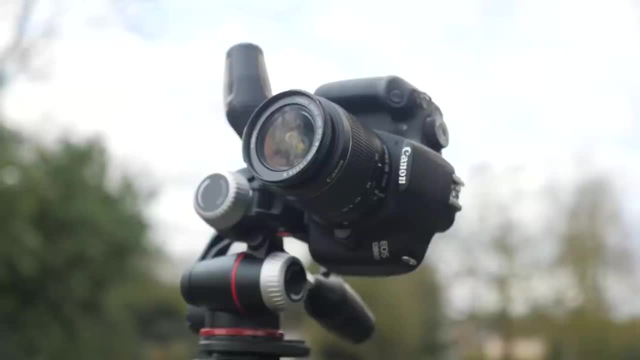 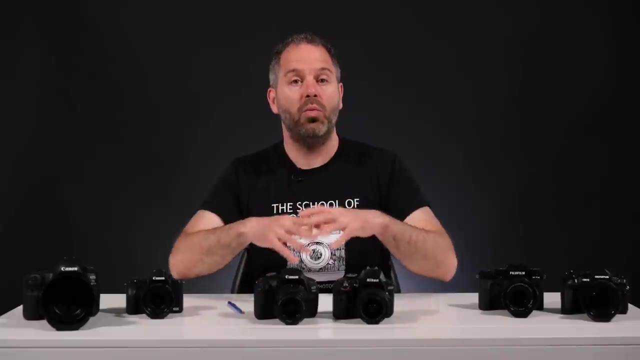 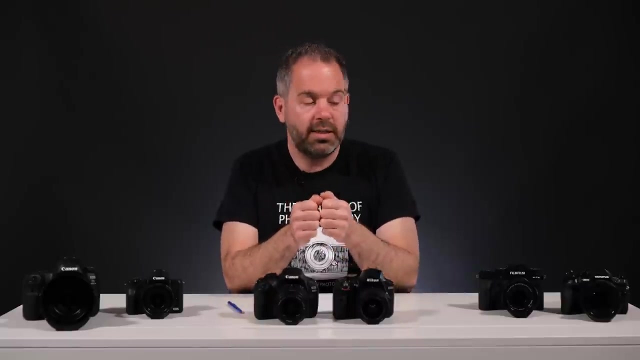 what you will need, though, is a camera that goes fully manual, and one that you can change the lenses on. then it's the size of the camera that you want to carry around with you. if size is really important- and what I mean by that is a smaller size- then 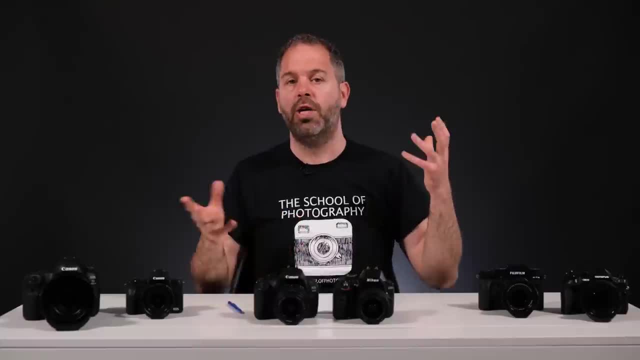 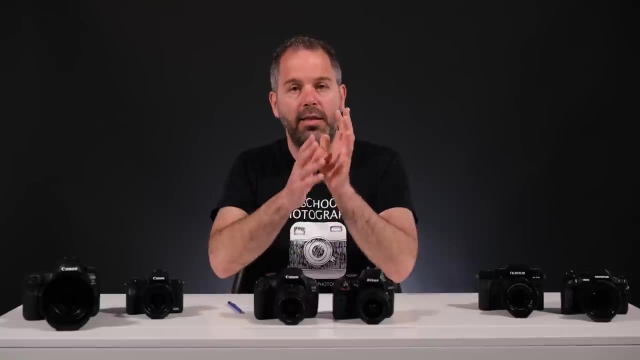 you're probably going to need to go for the micro four third range, because all the lenses are smaller, the cameras are lighter, the tripod will be lighter, Etc. if size is not a problem for you, then you know a crop sensor range or a full frame camera range. 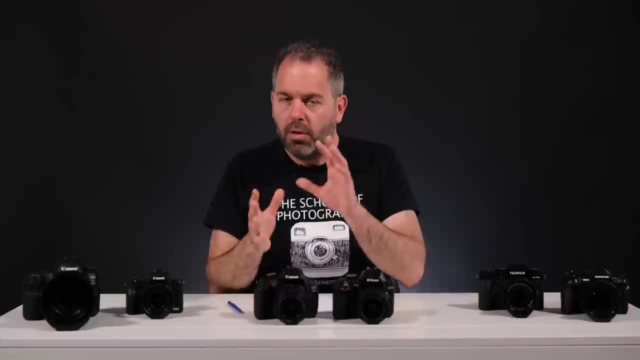 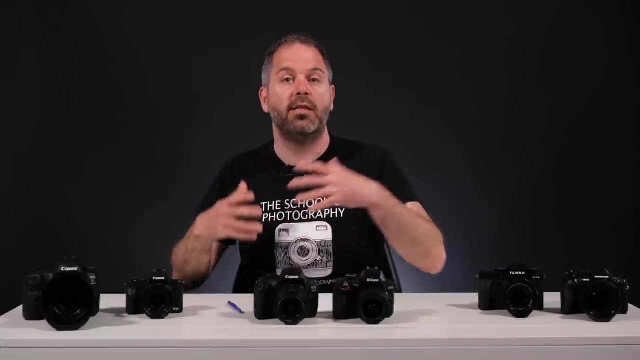 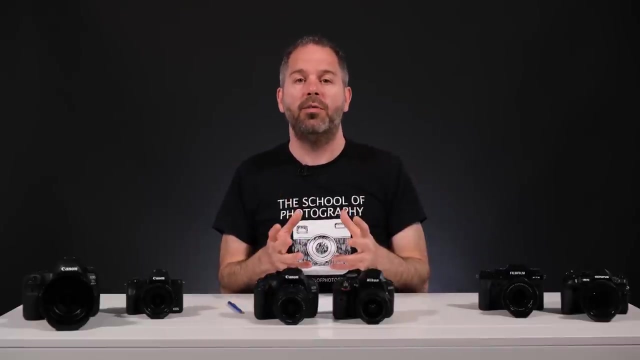 is going to be good for you as well. but what you do need to consider there is image quality over what you're going to use the pictures for. so, like I've said to you before, if you're not going to be shooting at high ISOs, you're not going to be printing really big. then the smaller sensor sizes: 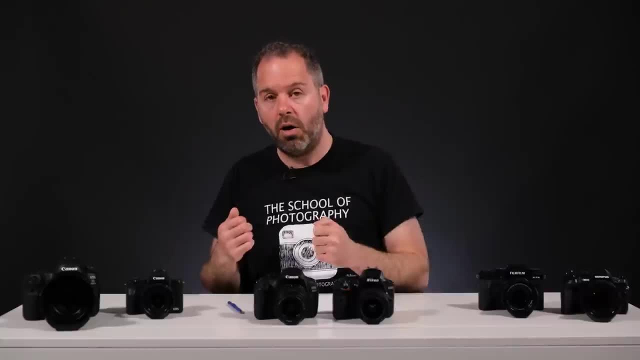 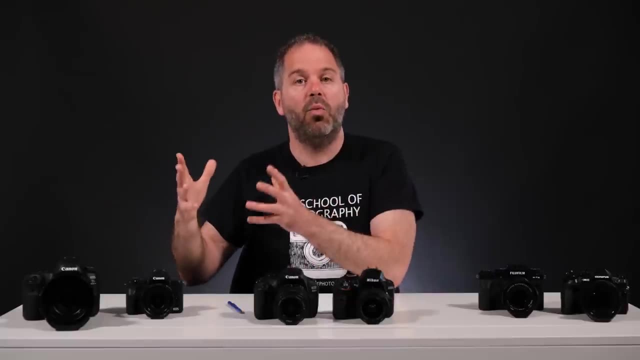 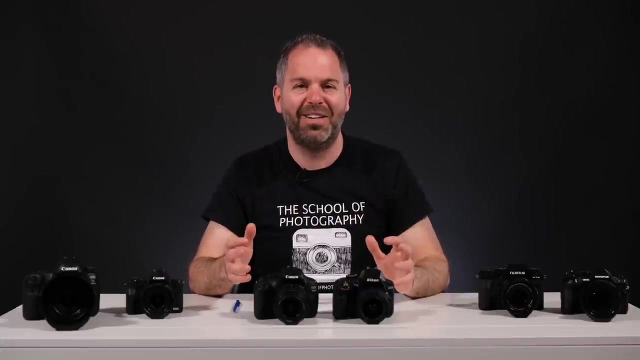 are going to be absolutely fine for you. if you are going to be printing massive, if you are going to be shooting at very high ISOs, then you're going to want to go for a larger sensor. or, of course, you go for a nice happy medium and you go for the crop sensor range, and then it comes to the brand that you choose now.